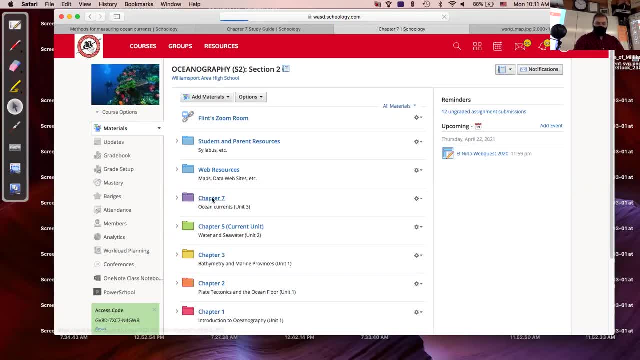 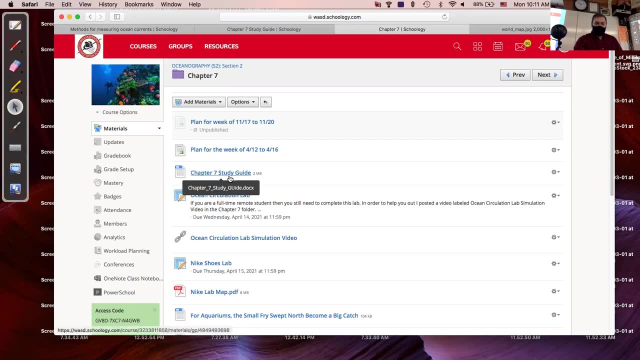 In the uh in the course in chapter seven, you'll find the uh chapter seven study guide. I give you a copy of it and I want to go over some stuff that's actually on the first two pages of the study guide. so if you have it, 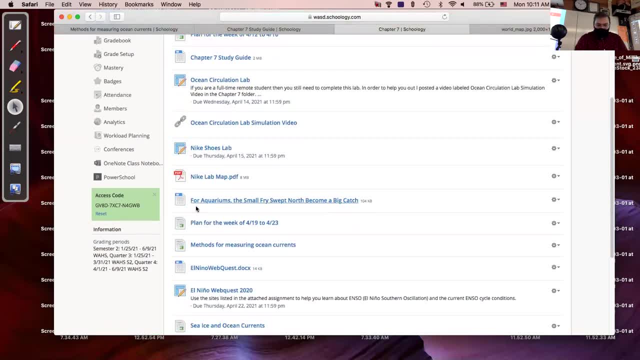 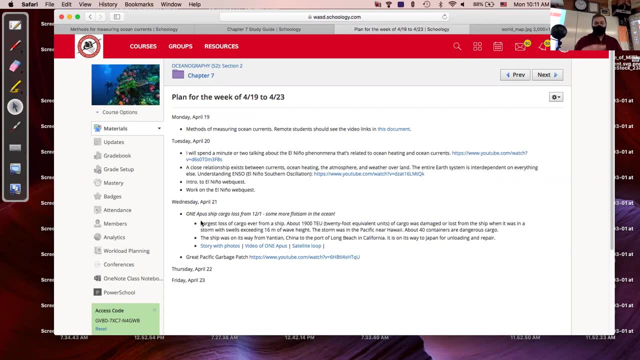 I can help you get stuff filled out so you understand stuff in the plan for the week. So I want to tell you about different ways that ocean currents are measured today and show you some good applications of that, and tomorrow I'll tell you some stuff about El Niño You may have. 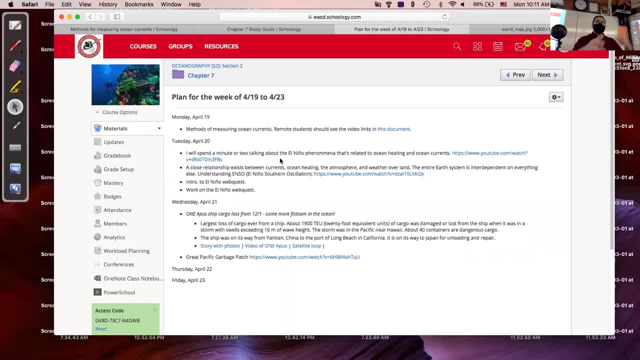 heard of El Niño as a uh like a weather slash climate thing. so there are changes in ocean currents that affect uh weather on a medium to long-term scale and we'll do some stuff with El Niño on Tuesday and Wednesday. and there's a thing about El Niño that's due on Thursday, I'll tell. 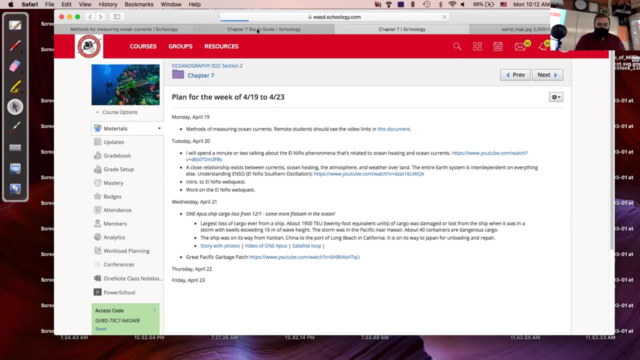 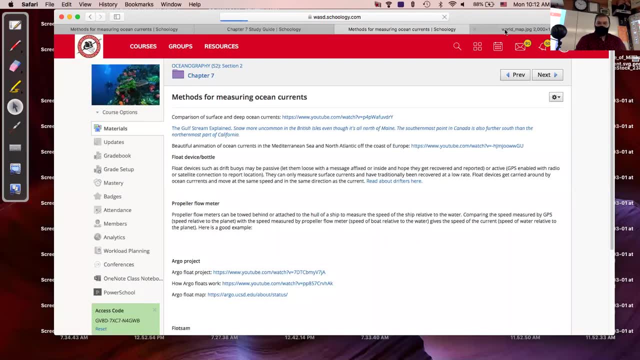 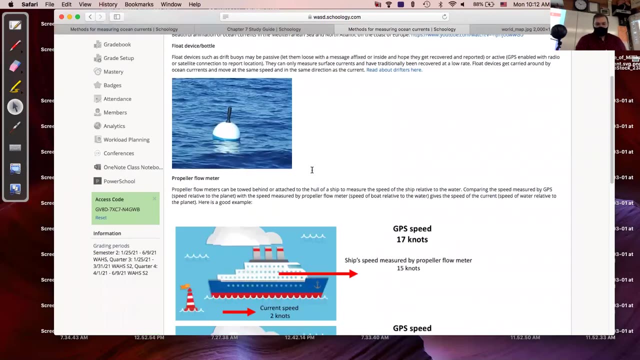 you about it tomorrow, Anyway. so if you're remote, I have some links here under the plan for the week. there's a thing that says methods for measuring ocean currents. This thing says methods for measuring ocean currents. there are a few different videos here, like this one and this one. it's best if you watch them like on your own, so in the chapter. 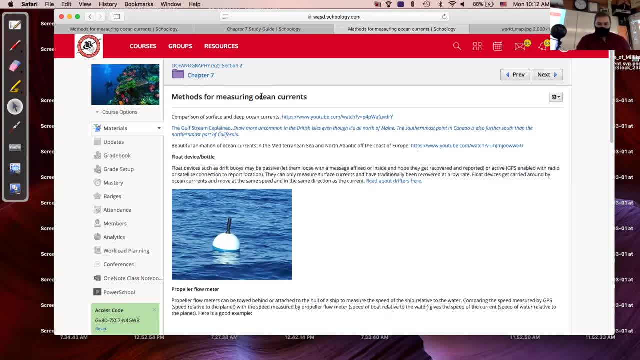 seven folder there's a thing says method for measuring ocean currents. So let me show you first about like ideas about surface currents and ocean currents. so if you're remote, that's a good link to follow there. I'll play it on the middle screen up here. sounds pretty good. I got some new speakers. they're pretty pimp. 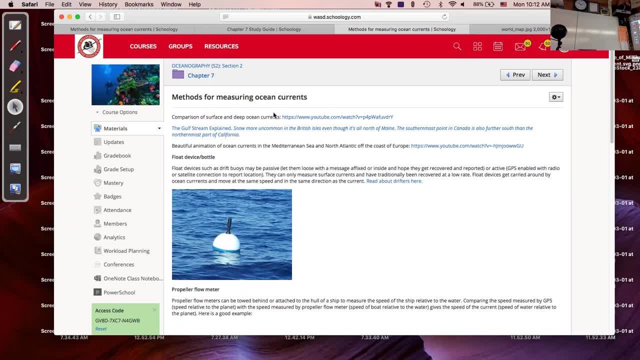 There's like an ad, but we gotta wait for the ad. yep, I actually want to be here, Okay, okay, At tech- Jong-in Library. Yeah, uh, I'll give you stuff tomorrow whenever it's good. presenter in computer. 1992, A cargo ship carrying bath toys got caught in a storm shipping. 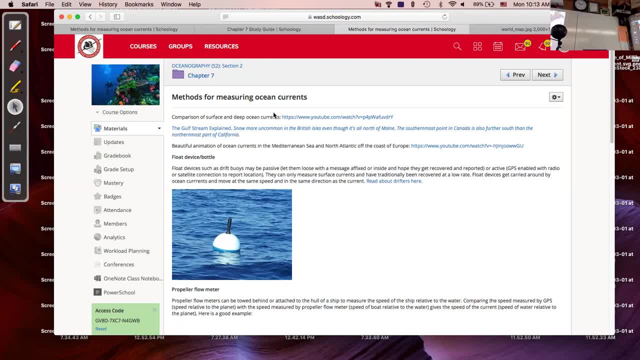 containers washed overboard and the waves swept 28,000 rubber ducks and other toys for a day into the North Pacific. But they didn't stick together. Quite the opposite. The ducks have since washed up all over the world, and researchers have used their 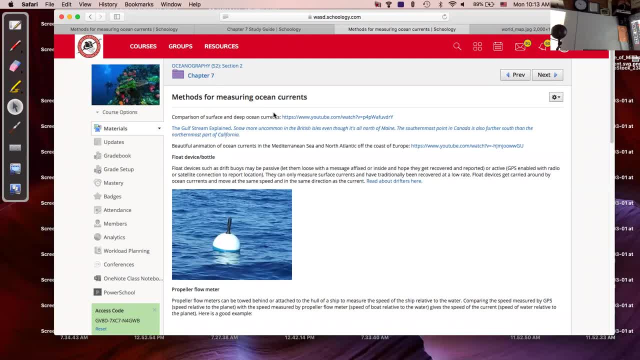 paths to chart a better understanding of ocean currents. Ocean currents are driven by a range of sources: The wind, tides, changes in water density and the rotation of the earth. The topography of the ocean floor and the shoreline modifies those motions, causing currents to speed up, slow down or change. 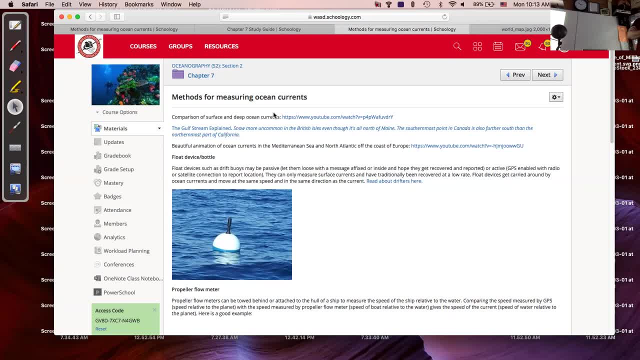 direction. Ocean currents fall into two main categories: surface currents and deep ocean currents. Surface currents control the motion of the top 10% of the ocean's water, while deep ocean currents mobilize the other 90%. Though they have different causes, surface and deep ocean currents influence each other in an 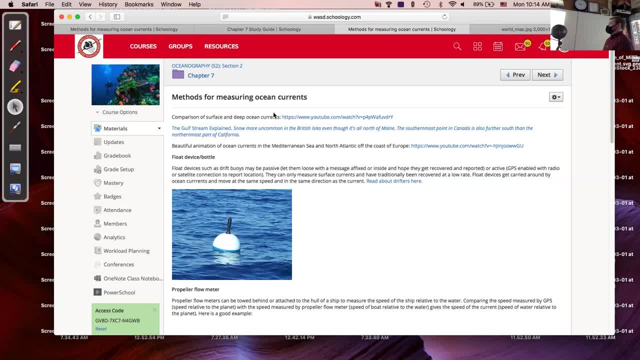 intricate dance that keeps the entire ocean moving Near the shoreline. surface currents are driven by both the wind and tides, which draw water back and forth as the water level falls and rises. Meanwhile, in the open ocean, wind is the major force behind surface currents. As wind blows over the ocean, it drags the 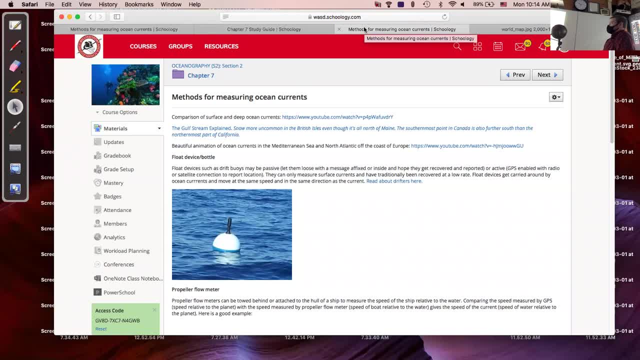 top layers of water along with it. That moving water pulls on the layers underneath and those pull on the ones beneath them. In fact, water as deep as 400 meters is still affected by the wind at the ocean floor. Although the Earth's rotation went up a bit earlier, some of its currents are 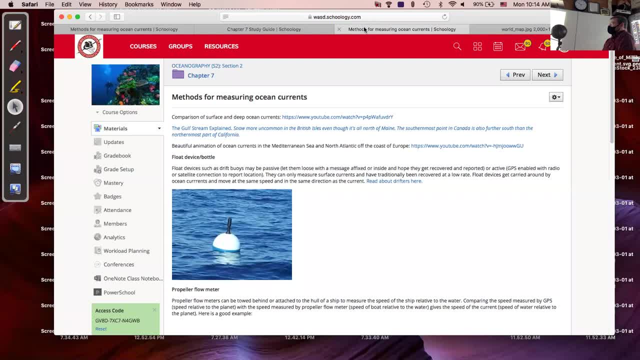 pretty similar to those of the ocean's water surface. since air and water move back and forth at record lows, There is a common德, And the earth's rotation still affects the wind patterns that give rise to these currents. If the earth didn't rotate, air and water would simply move back and forth. 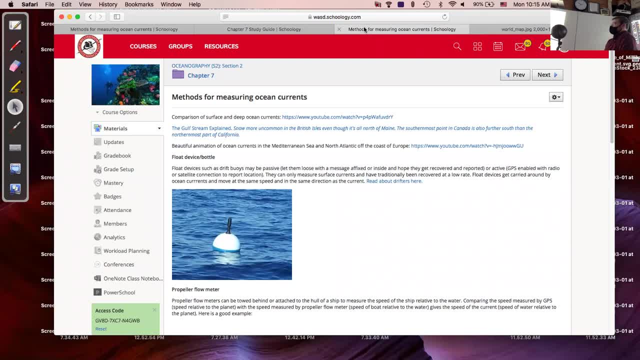 between low pressure at the equator and high pressure at the poles. But as the earth's rotation turned, the wind currents would rise. This is the way the earth's rotation was formed, and the water would just move back and forth between the low pressure at the equator and high pressure at the poles. But now? 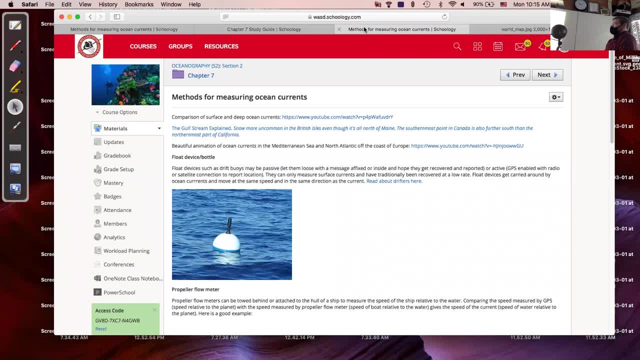 as the earth's rotation around us- it's available on the Earth- spins. air moving from the equator to the north pole is deflected eastward, and air moving back down is deflected westward. the mirror image happens in the southern hemisphere, so that the 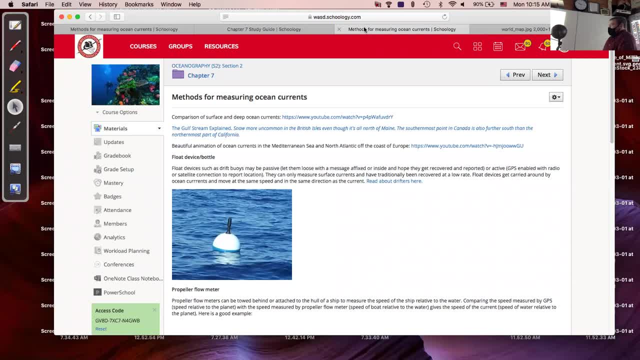 major streams of wind form loop-like patterns around the ocean basins. this is called the coriolis effect. the winds push the ocean beneath them into the same rotating gyres and because water holds on to heat more effectively than air, these currents help redistribute warmth around the globe. unlike surface currents, deep ocean currents are driven primarily by changes. 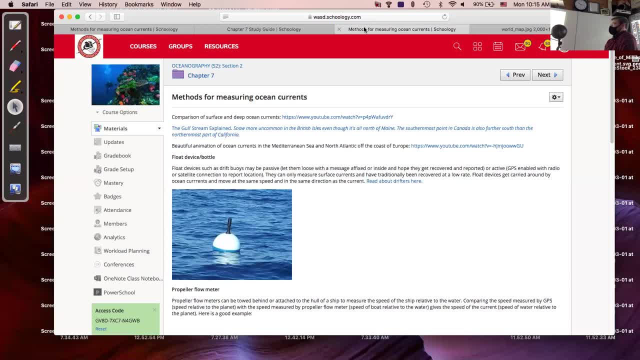 in the density of sea water. as water moves towards the north pole, it gets colder. it also has a higher concentration of salt because the ice crystals that form trapped water while leaving salt behind this. cold, salty water is more dense, so it sinks, and warmer. salt water is more dense, so it sinks and warmer. salt water is more dense, so it sinks and warmer. 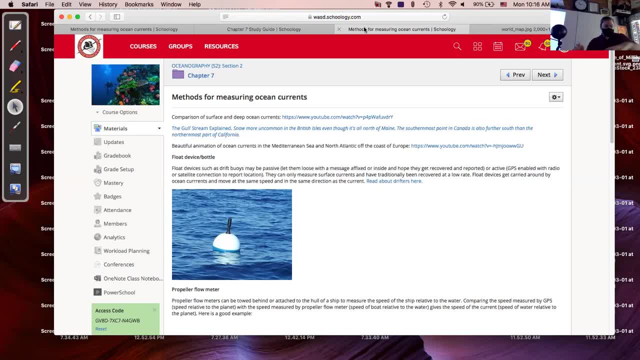 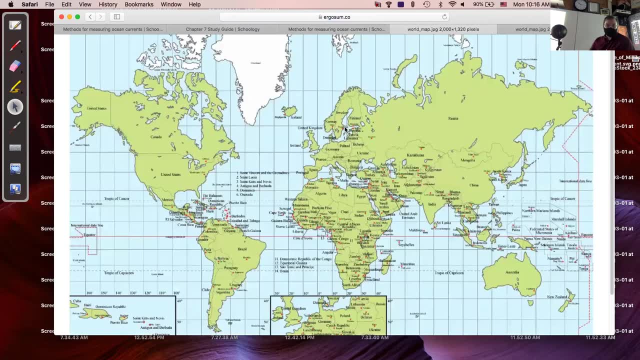 surface water takes its place, setting up a vertical current called thermohaline circulation. thermohaline circulation of deep water and wind-driven surface currents combine to form a winding loop called the global conveyor belt. as water moves from the depths of the ocean to the surface, it carries nutrients that nourish the microorganisms which form the base of many ocean. 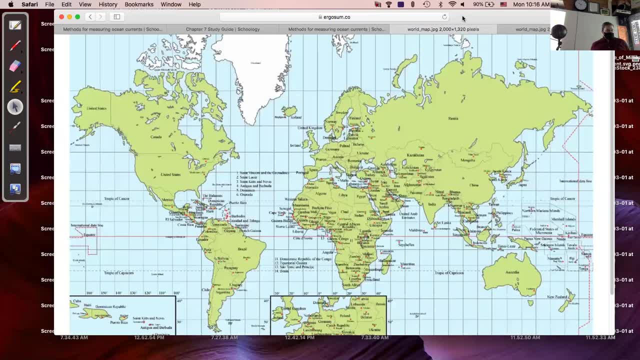 food chains. the global conveyor belt is the longest current in the world, snaking all around the globe, but it only moves a few centimeters per second. it could take a drop of water a thousand years to make the full trip. however, rising sea temperatures are causing the conveyor belt to 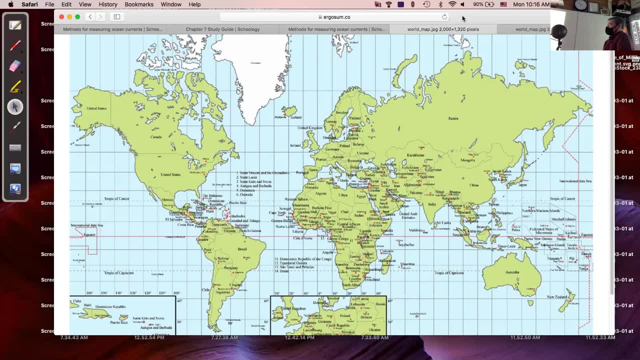 seemingly slow down. models show this causing havoc with weather systems on both sides of the atlantic, and no one knows what would happen if it continues to slow or if it stopped altogether. the only way we'll be able to forecast correctly and prepare accordingly will be to continue to study the 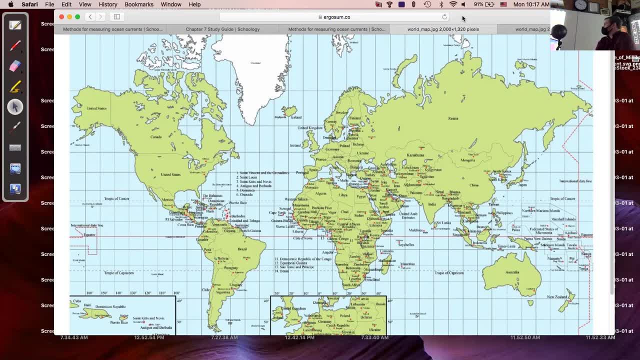 currents and the powerful forces that shape them. what about? all right, so the next one i want to show you is actually about, uh, the gulf stream, so a specific current that's important, um you've already seen some stuff about, is this gulf stream current, which flows, uh, from, really, the southern? 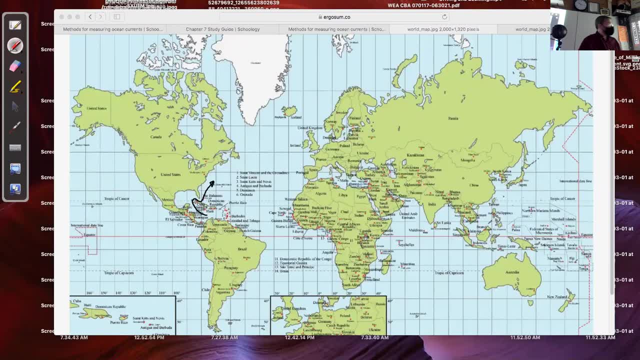 caribbean, up through the gulf of mexico and up along the eastern united states, but it continues, uh, across the atlantic ocean and up to northern europe. so here's a thing a bit of like geography trivia. if you draw a line, this line of latitude, right here, let me, uh, i can get a straight line. 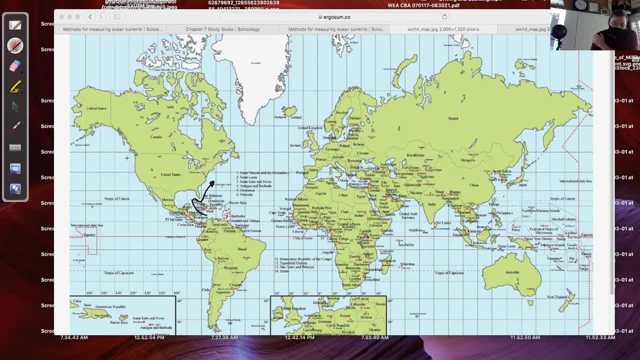 on this thing. oh, my straight line tool's not on there anyway. see this line of latitude. you draw this line of latitude straight across. every part of the continental united states is below that line, but all of england is above that line. most of england, the british isles, is the same latitude. 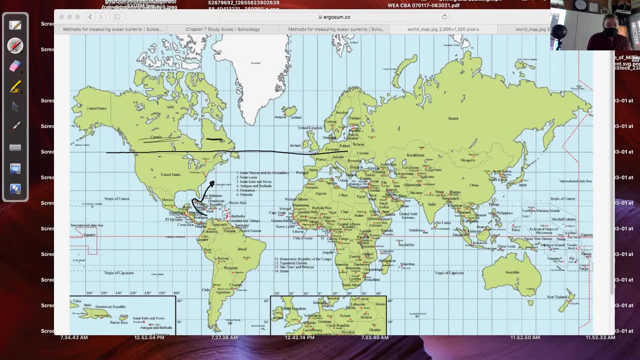 as much of like central quebec and ontario and the central canadian provinces. when you think of england, you probably don't think of like heavy snow, storms and really cold winters. that's because they don't have them. it can snow in england and they do get snow from time to time. 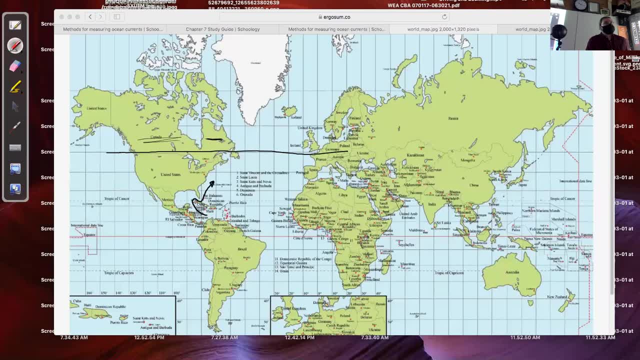 but it's not particularly cold like it's a. you know they get a lot of rainfall but they don't have really really, really super cold winters. but even you know, down into the in the appalachian mountains, well down into west virginia and virginia, you can get heavy snowfall in the wintertime. but very, very 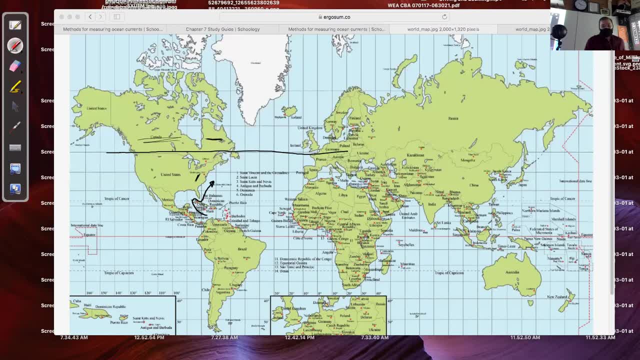 infrequent snowfall uh in the british isles, and it's mostly, it's in large part because of this gulf stream current which carries warm water not only up along the east coast of united states but all the way across into uh like england. so england, ireland, scotland, okay, so if you are remote, if you, 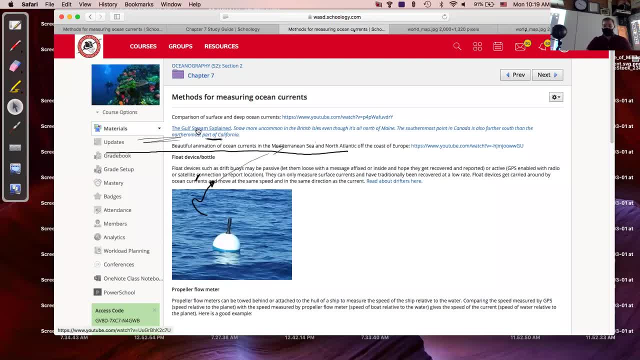 this next one here- the gulf stream explained- that's the one i'll show now because it has to do with- so keep that in mind- about the role that that gulf stream plays with, uh, europe. so this, this video, is actually made for audiences in europe, but it's you know. 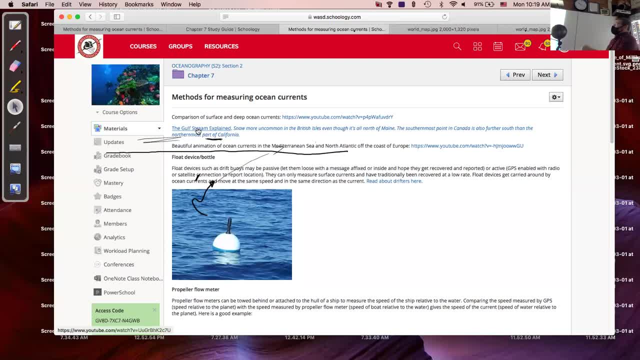 completely makes sense on a global scale. oh, there's an apple event. what's it gonna be? the ocean conveyor belt and the gulf stream: ocean currents have a direct influence on our lives. they determine our weather, our climate and much more. the ocean currents and wind systems transport heat from the equator to the poles. 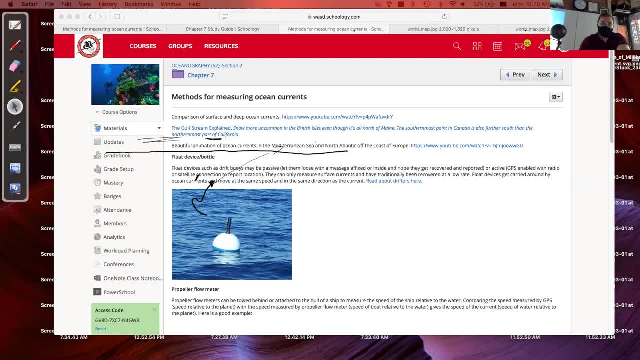 and operate like a large engine for the global climate. in the oceans there are numerous currents. the so-called ocean conveyor belt is very important for our climate. this term describes a combination of currents that result in four of the five global oceans exchanging water from each other. they form a worldwide circulation system. 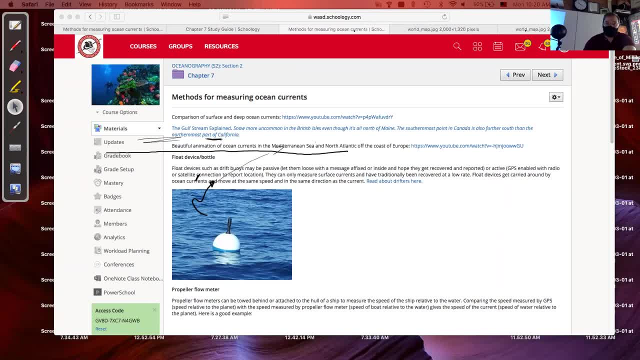 the conveyor belt is also called the of haline circulation, with thermo referring to the temperature, and halide to the salt content of the water. both determine the density of the water. while the masses of water may be moved in part by wind, primarily the different densities of the global oceans are responsible for their movement. 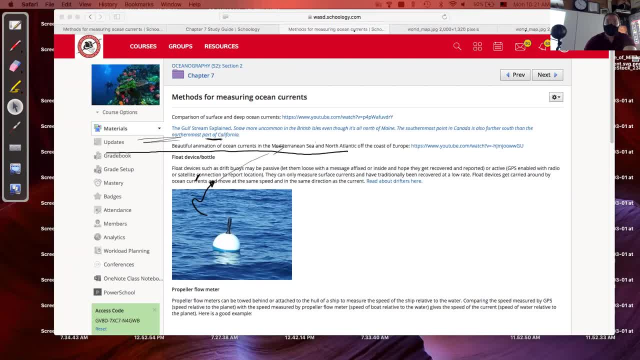 warm water has a lower density and measure of the hollow. it will show us a whole host of other wonderful things about the ocean rises while cold water sinks. The water's density also increases with a higher salt content. At the equator, the heat from the sun is especially strong, resulting in a lot of evaporation and thus 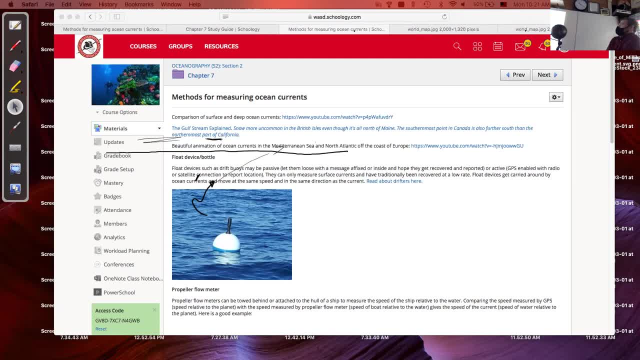 a rise in the water's salt content. That is where the Gulf Stream begins. The Gulf Stream is very important for the European climate. Its length of 10,000 kilometers makes it one of the largest and fastest ocean currents on Earth, and it's very warm. At roughly 2 meters a second, it brings up to 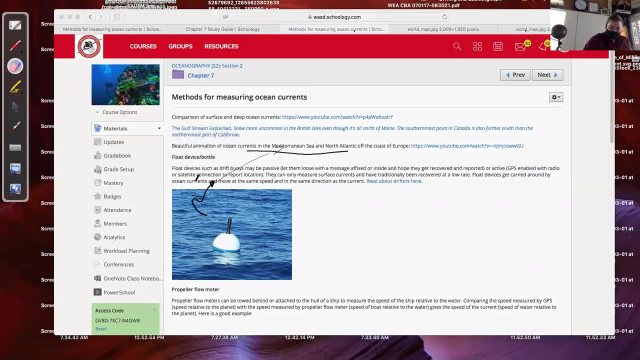 100 million cubic meters of water per second towards Europe. A constantly blowing wind- the southeast trade wind- drives warm surface water to the northwest, into the Gulf of Mexico, where it heats up to 30 degrees Celsius. The turning of the Earth. and the west winds then direct the Gulf. 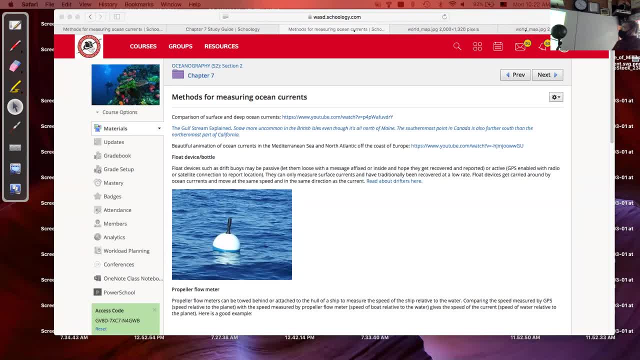 Stream towards Europe and split it up. One part flows south, another east, to the Canary Current, and a third part flows north, where it releases a lot of heat into the atmosphere. as the North Atlantic current, The water becomes colder there, Its salt content and density rise on account of evaporation and it drops down between 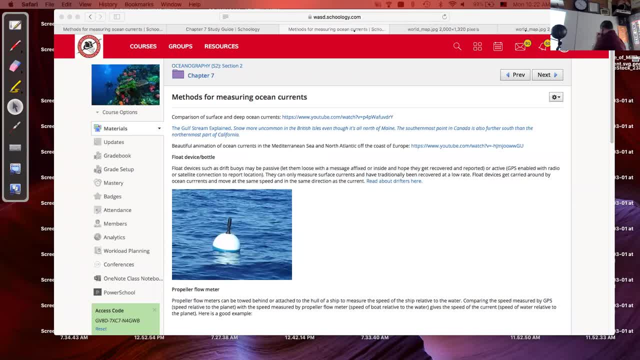 Greenland, Norway and Iceland. There we also find the largest waterfall on Earth, roughly 15 kilometer wide. The Gulf Stream is the largest in the world, with water falling up to 4,000 meters. It's 17 million cubic meters of water per second, or roughly 15 times more water than is counted by all the rivers in the world. 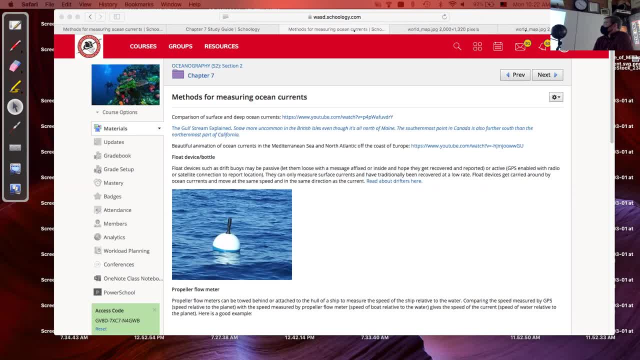 The Gulf Stream is a strong well strong, which constantly pulls in water. The reason that the Gulf Stream moves towards Europe: The Carolus species use the Gulf Stream as a means of transport on their troops from the Caribbean to northern areas. It doesn't just bring us animals, but it also brings us people. 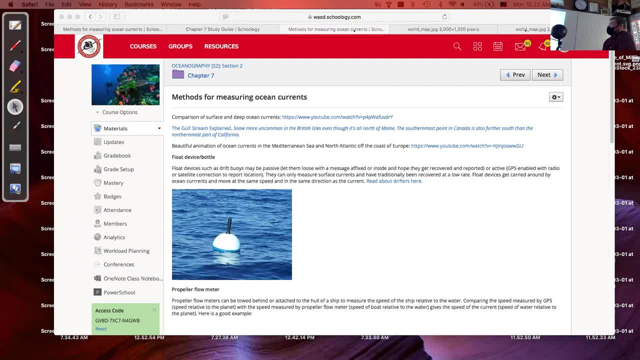 The Gulf Stream also comes with it. In order to reduce the same heat which it brings to the shores of Europe, we would need one nuclear power plant. That's why we also call the Gulf Stream a heat pump. Without it, the temperature would be significantly. 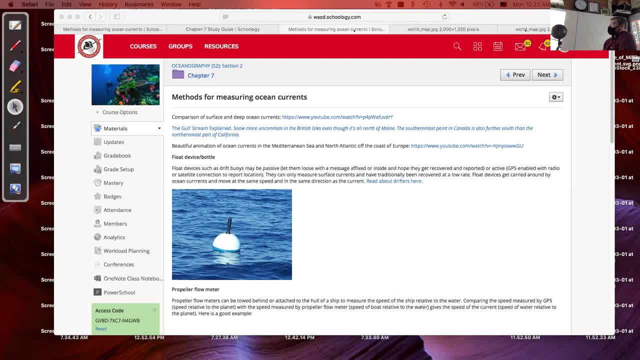 colder here, at least 4 to 10 degrees. Instead of lush fields, we would have long winters and sparse, ice-covered landscapes in Europe. In the last few years, scientists and pundits in the media have repeatedly expressed the fear that the Gulf Stream could come to a standstill due to climate change. 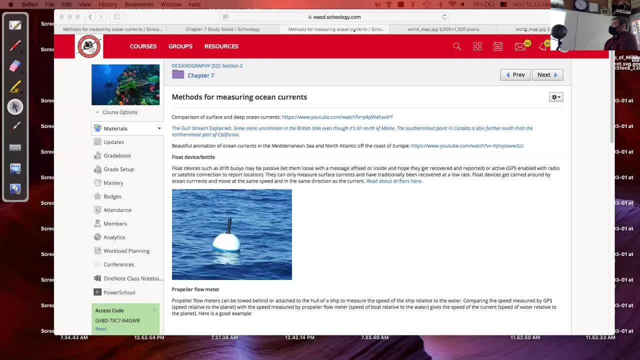 Because if the polar caps actually melt, the salt content in the water off Greenland would fall, as would its density. The North Atlantic would no longer be heavy enough, and that's so it wouldn't sink as usual. In the worst case, that would bring the Gulf Stream, our heat pump, to a stop. 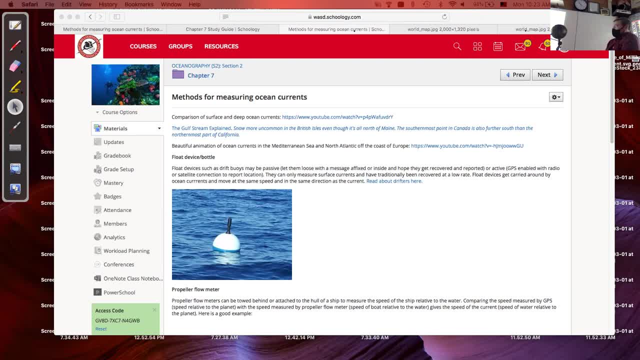 Some climate experts also assume that climate change could compensate for this effect. We know that it can be normal for the climate to change by changing the climate. We know that it can be normal for the climate to change by changing the climate. We know that it can be normal for the climate to change by changing the climate. 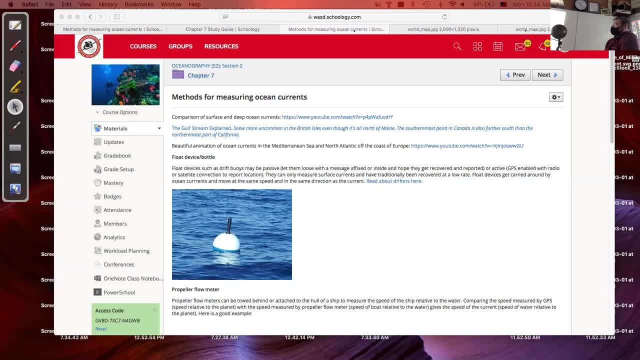 We've been looking at the development of the Earth over the last few million years. There are risages and warm periods. In the last ice age, a gigantic flood of melting water crippled the Earth, involving North Atlantic current covering the northern hemisphere in ice. 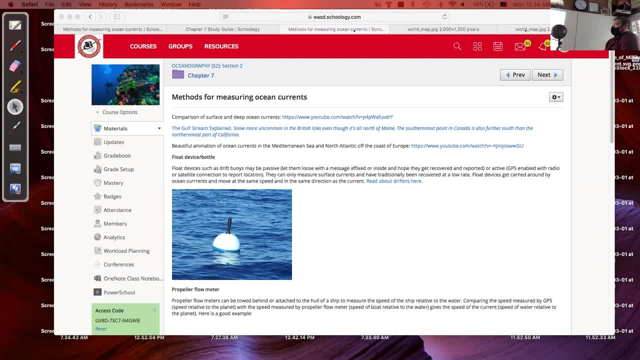 Scientists have different views on the impact that climate change will have on the global ocean. compared to мер-belt. One thing is clear: When the climate changes, then the complex system of dosage, currents and winds- and winds, which has remained fairly stable since the last ice age, will change in ways that we don't. 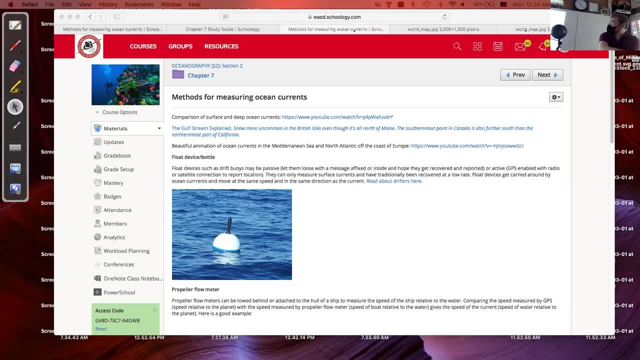 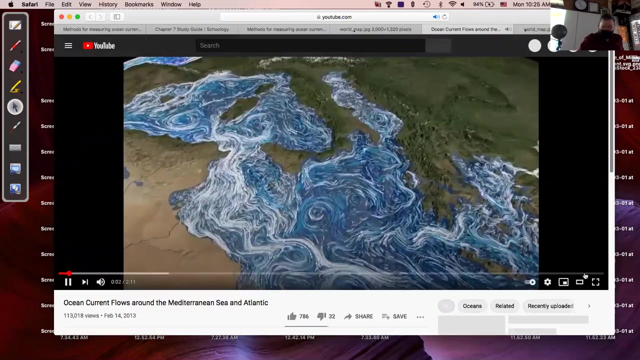 yet understand, okay, and then, uh, let's see there's a really, really, really excellent animation. it's the next link and the thing will be on both the side screens about, uh, relative ocean currents in, in and around europe and the mediterranean. so this is the mediterranean sea here. this is the 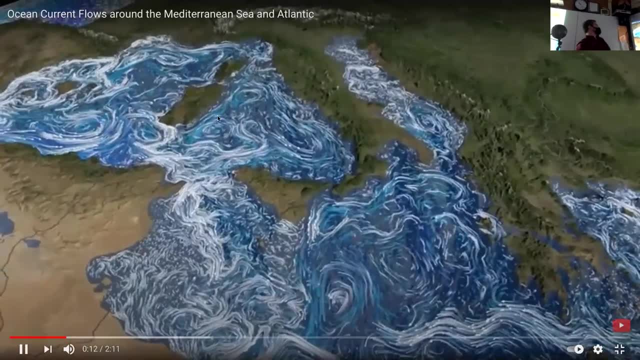 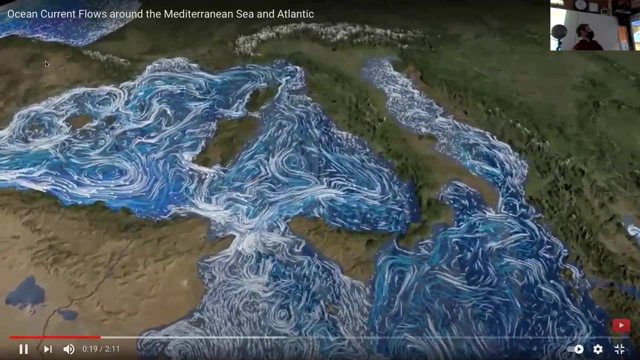 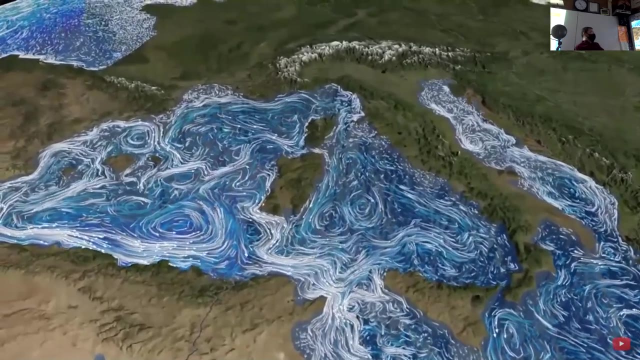 southern part of italy, the boot of italy, and then, uh, this is the main mediterranean sea. this is, uh, france, up here, francis here, spain is there. so you can see, the motion of the currents can be very complex. within, uh, with an ocean basin, there's a general flow. 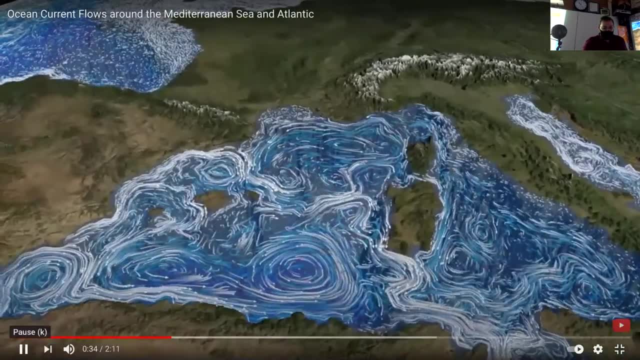 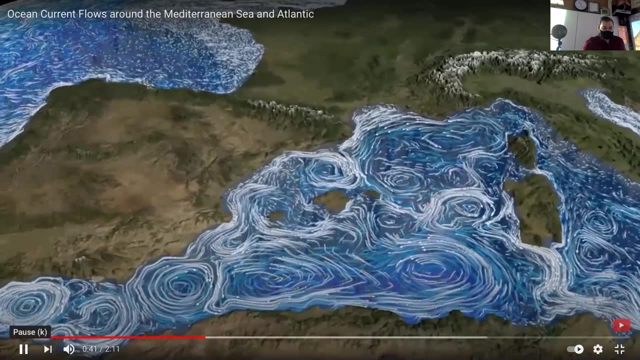 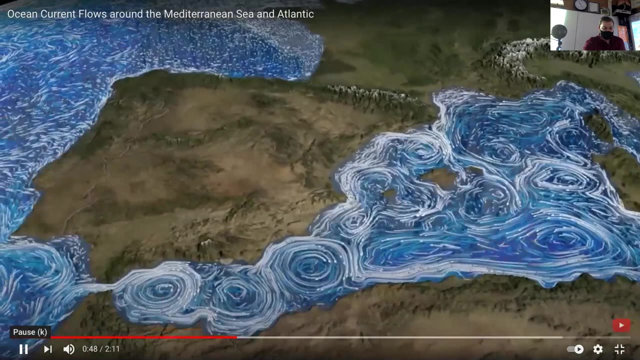 of water into the mediterranean sea through the strait of gibraltar. so you may know, let's get to it all right. so next song: again, this is portugal here, and i think this is united states. uh, this is so i've got to go ahead and just get to this one. 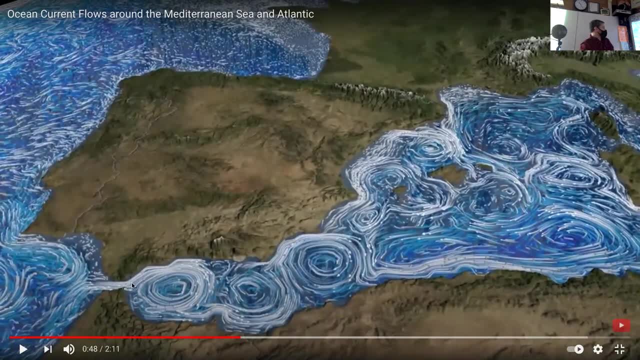 string and bring it back to. it's the five states, and i have one more. i think so. the five states are, and this is Spain, this is Northern Africa. water flows into the Mediterranean Sea through the Strait of Gibraltar. He's like sawing a log. 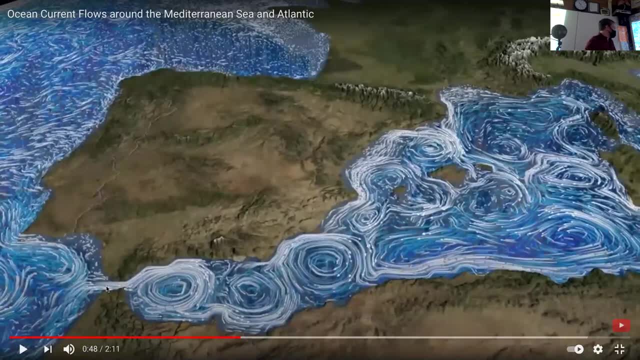 He's like hear him Pretty good, Anyway. so water flows in and then it forms these gyres. A gyre is a localized current where there's a motion as a result of differences in topography and whatnot, And then that water 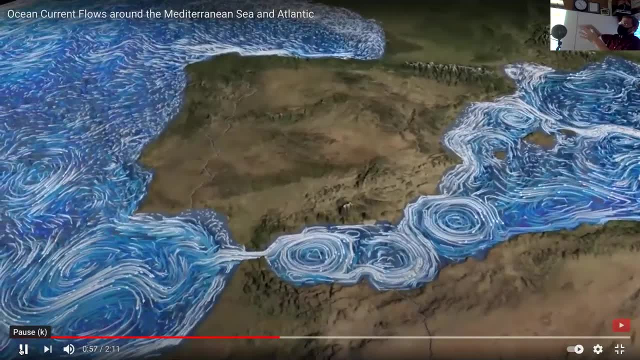 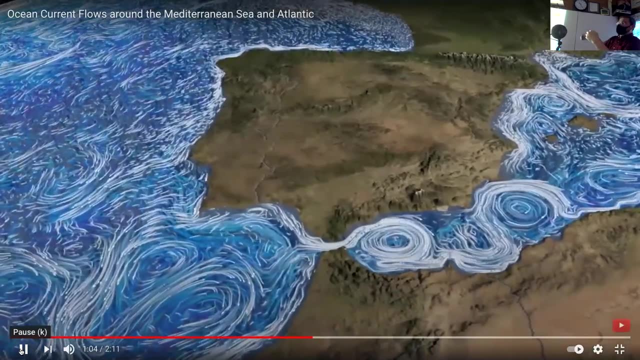 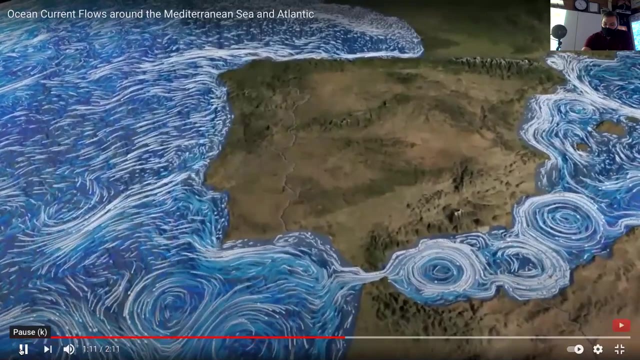 when it flows into the Mediterranean Sea. there and then that could be from tidal action and it can flow back out. but it can also flow out of the Mediterranean and into the Indian Ocean through the Suez Canal And places where there are restrictions oftentimes have very, very high current speeds. 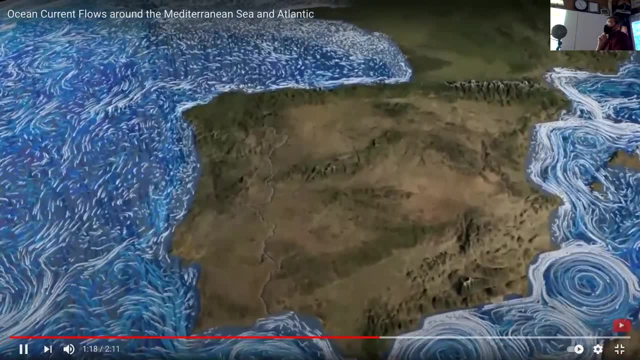 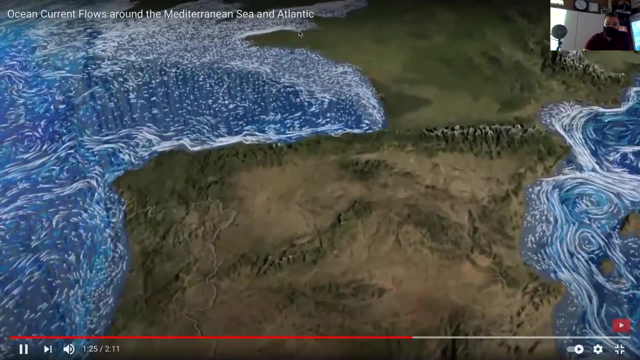 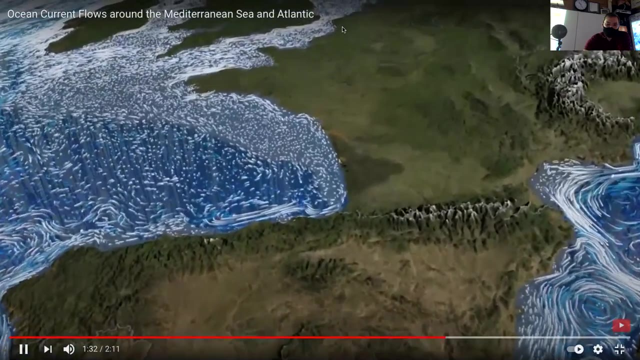 So another place that has a very high speed of current is the English Channel And the English Channel's current changes direction. So up here between France and the British Isles you'll see the density of the lines goes way up And the direction of that current changes. from heading north to heading south, depending upon the time of the month and the direction of the tides as a result of the pull of the sun and the moon. So there it's a northerly path, and then it changes and it's a southerly path. 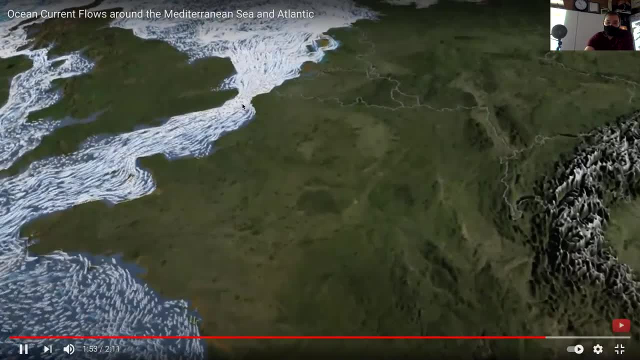 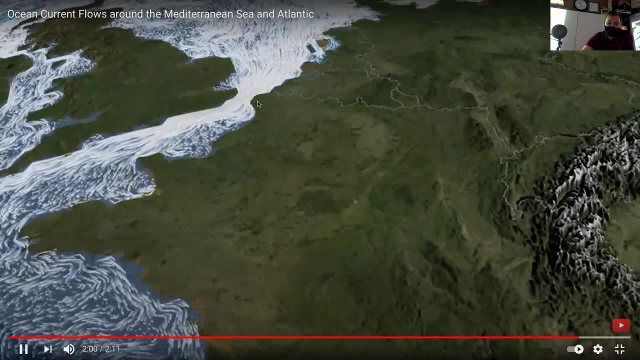 But the speed of the water through this narrow English Channel here can be very, very, very high in one direction or another And sometimes it's like a slack speed or like slow. So you know, the distance from England to France isn't that great across this channel. 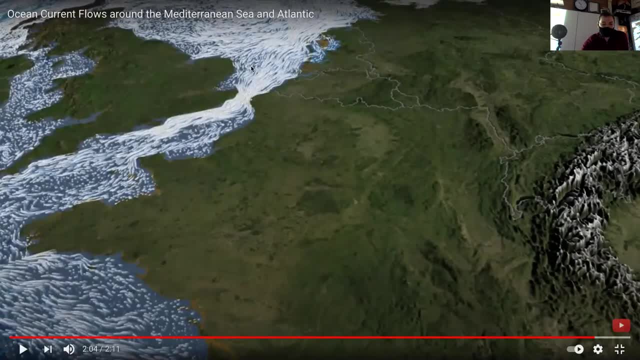 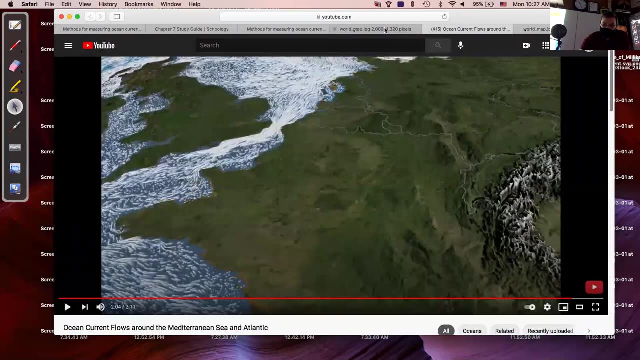 It's a relatively narrow passage. Lots of shipping takes place through there And then, I don't know, in the history of World War I and World War II it was very important. So let's see. So the major devices for measuring ocean currents. 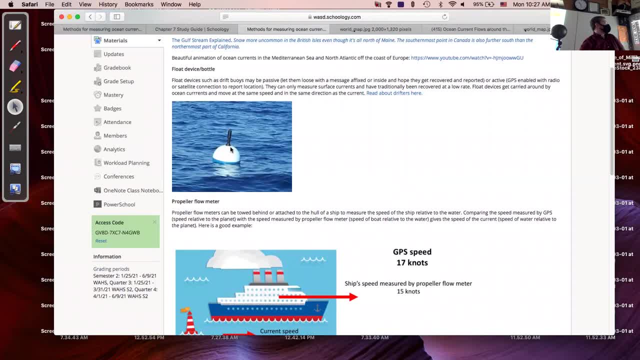 include measuring the motion of a thing that's floating in the water. So sometimes it's intentional, sometimes unintentional, But the unintentional things, like the Nike shoes or the rubber duckies. it's kind of fortunate to oceanographers that we can study the motion of the path of those things. 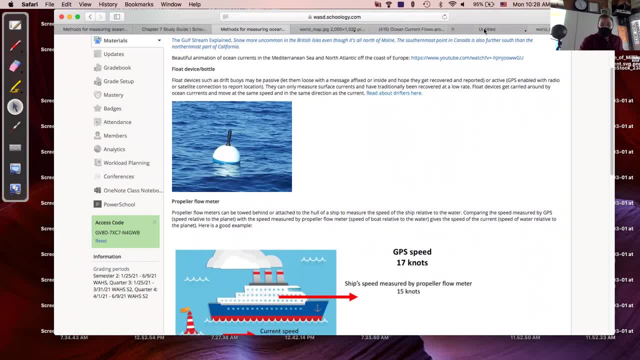 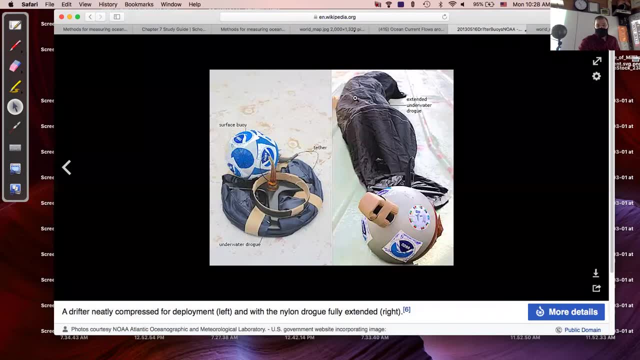 But we also build intentional drift buoys, And those drift buoys aren't just dumb things that you put into the water Oftentimes. this is a good example of a NOAA drift buoy: There's a big plastic bag which hangs down into the water. so that you're mostly measuring the motion of the water And not measuring the effect of the wind blowing on it. And then oftentimes you're not just you're gonna measure the position, but you can also measure the salinity and the temperature. 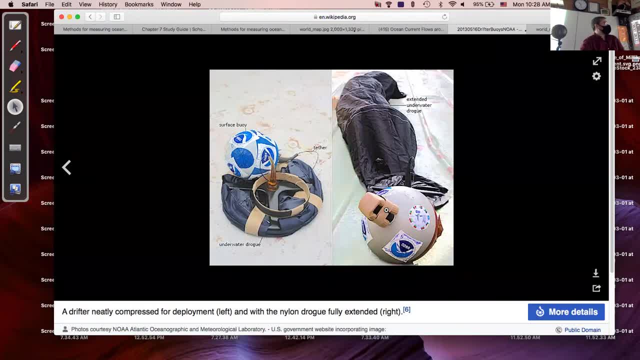 maybe the pH of the water, And then up here be able to send location, temperature, salinity, maybe pH information by radio to a radio receiver, either for a passing ship or up to satellite, And then you can also recover the thing later. 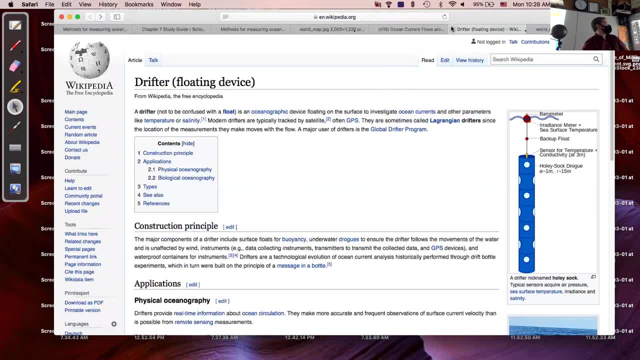 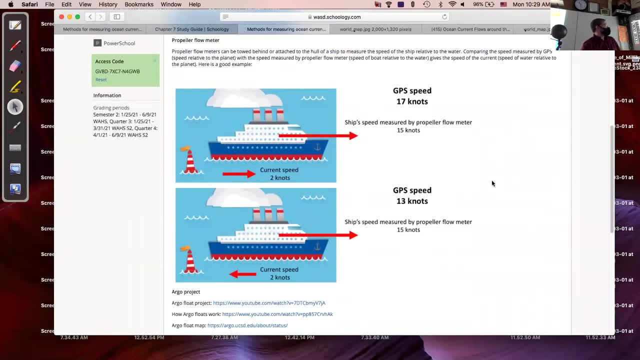 So the traditional method of measuring the motion of currents is to like throw something in the water and see which way it goes. Another common way that current speeds are measured is actually done through shipping. industry And the Navy has done this technique and it's a very common technique. 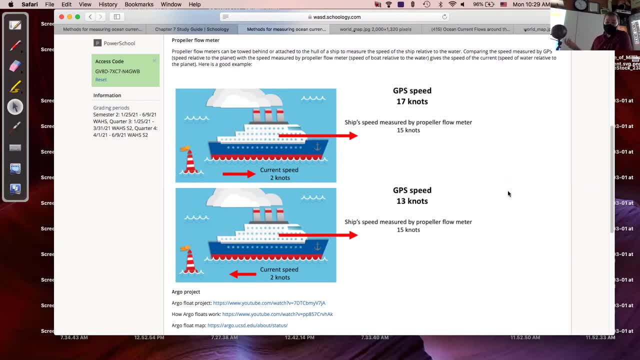 both in shipping with boats and also with aviation, to figure out the speed of the wind or the speed of the water And compare the speed of the boat relative to the water to the speed of the boat relative to the planet. So, for instance, here's a ship. 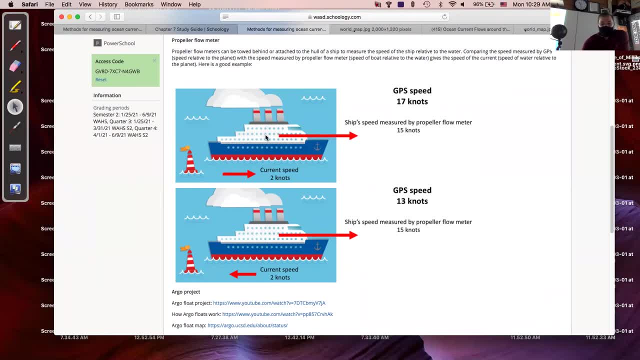 maybe like a little cruise ship, and the cruise ship is moving along And the propeller is propelling the ship in the water with a speed of 15 knots. So a knot is a speed that's about 1.2 miles per hour. 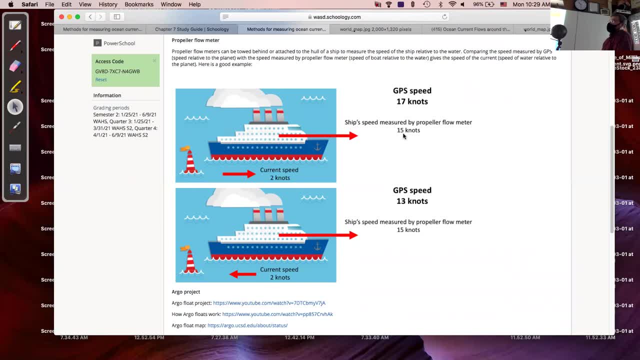 Knot is a common unit of speed used in both aviation and in navigation by ship. So the boat thinks it's going 15 knots in the water, but whenever you use a GPS to measure the motion of the ship, the GPS says you're going 17 knots. So if you're heading in this direction in the water and your speed relative to the water is 15 knots but the GPS says you're going 17,, it's as if you've got like a two knot kind of like boost or advantage. 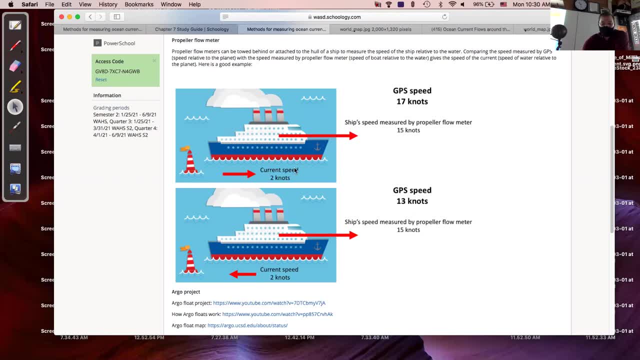 And that must be because the water itself is moving, maybe with a speed of two knots. So, in other words, if you were to shut the propellers or the ship off, shut the engines off, the ship would still drift along with the current. 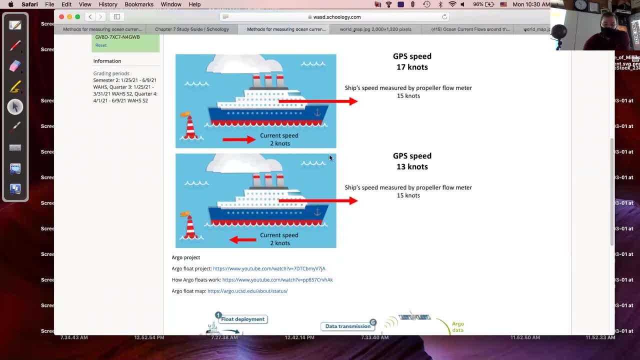 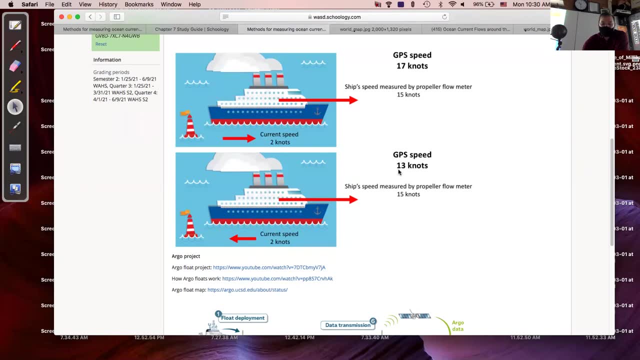 at a speed of two knots and you don't even have to do any work. On the other hand, if the ship is steaming along with a speed relative to the water of 15 knots, but a GPS says that you're moving 13 knots, 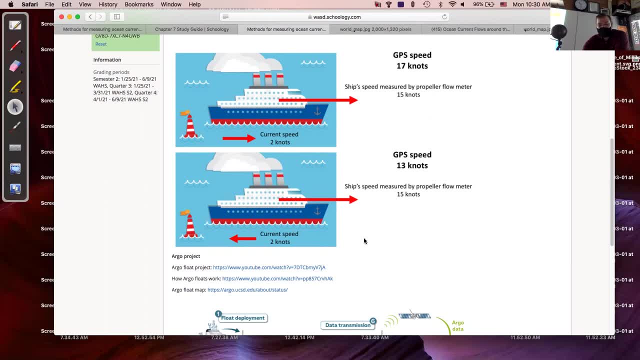 relative to the planet. it must be, because the current is heading in the opposite direction. So whether you're going into or away from a current that's two knots has a significant different, has a significant effect on the speed of that ship If you're going in the same direction as the current. 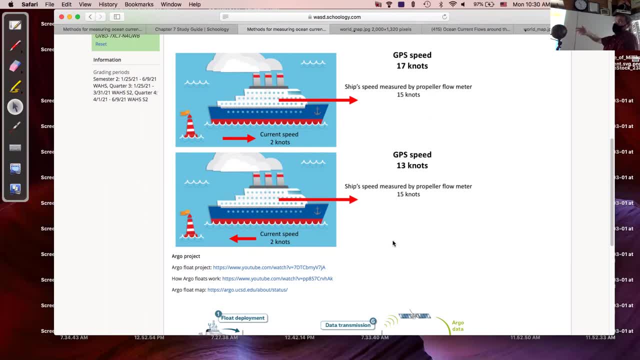 now you're going 17 instead of 15.. If you're going the opposite direction, it's 13 instead of 17.. And going 17 instead of 13 is a huge difference in speed and can give you a big advantage in time. 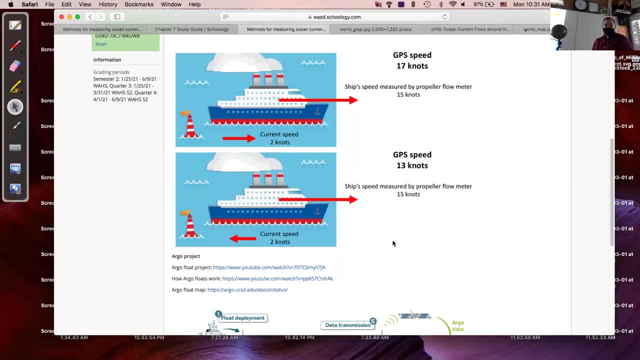 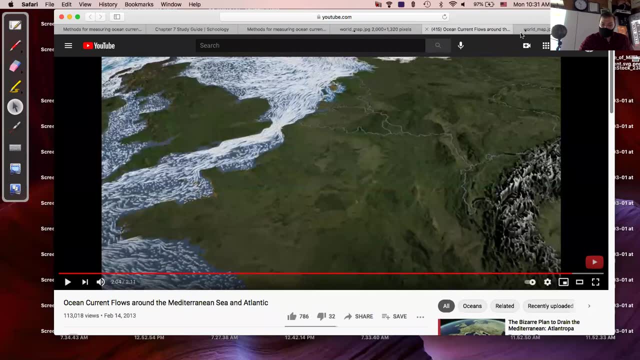 if you're trying to go all the way across the world's oceans. So lots of issues with navigation in plotting courses are as a result of dealing with currents. So, for instance, if you're like, okay, I'm gonna maybe leave New York and maybe sail, 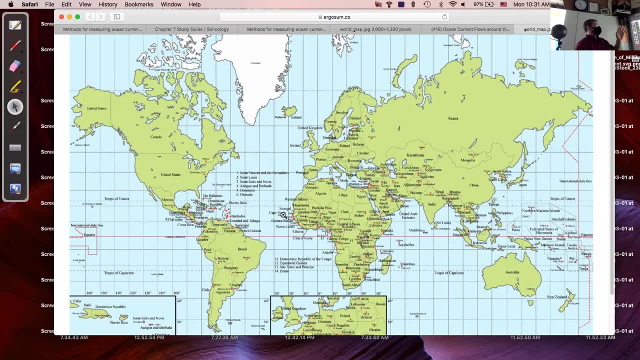 to Cape Verde, maybe not sail, not a sailing boat, but a motor yacht, and you're gonna travel from one place to the other, like when Jayden buys his like yacht on whatever site, that is, If, as you travel from one place to the other. 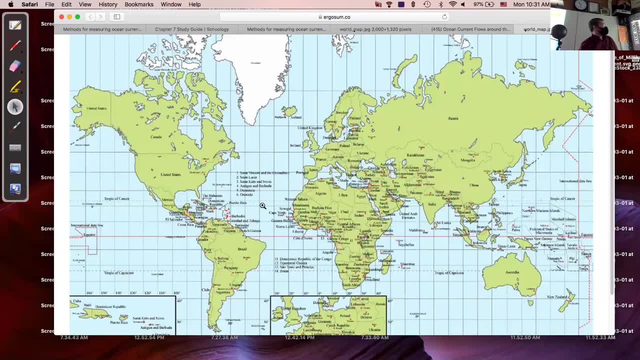 if the current is heading in the same direction, in the direction you're traveling, it will reduce your travel time. But if, on the other hand, the current from Cape Verde back to, like, New York is heading in that direction, you'd wanna avoid the current. 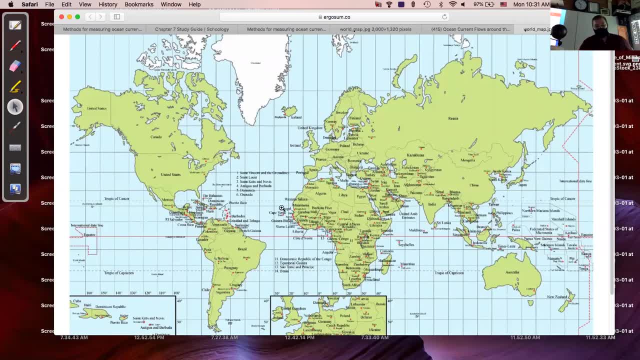 by maybe taking a more circuitous path so that you're not directly in the current or find a current that's going in the same direction. In a way it's like a conveyor belt. It can help you with navigation and travel. So it turns out that to oceanographers, 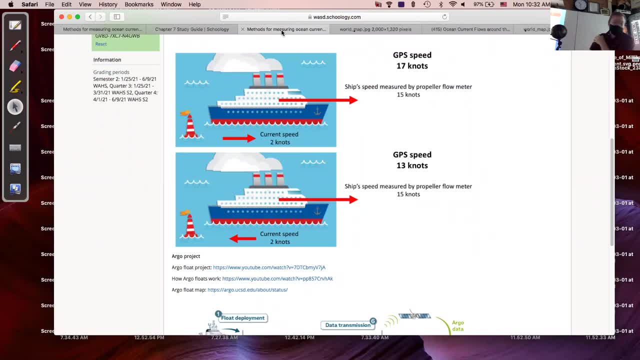 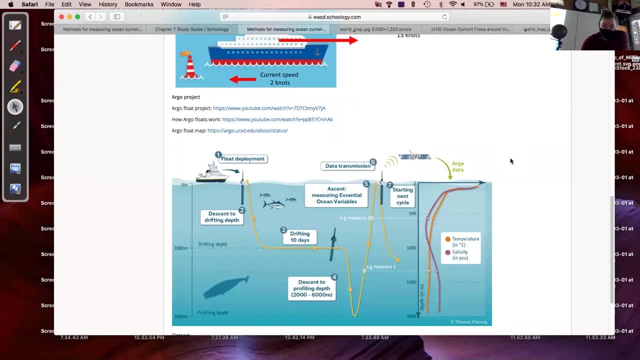 it's very useful to learn about ocean currents for a lot of different reasons, but the practical way we know about the world's ocean currents and how we've measured them historically is from trying to save time and money in shipping stuff around the world. Okay, another way to measure ocean currents. 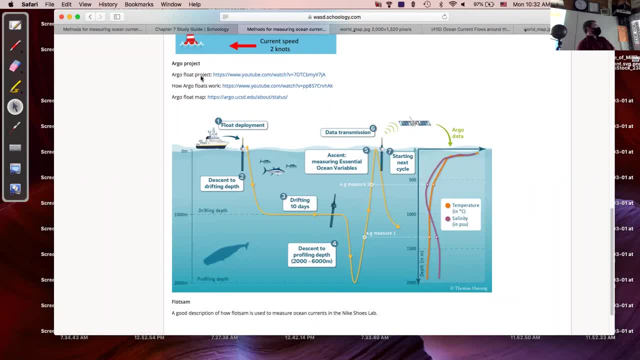 that's more sophisticated is a project called Argo. So here's an issue: When you put a float on the surface of the ocean, the only thing that you're measuring is just the speed of the water at the surface. But, like in the videos, and what's true, 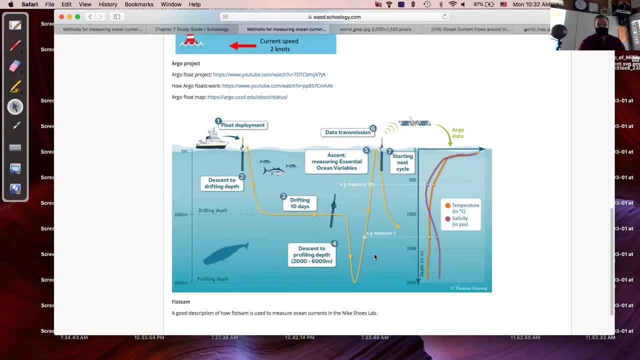 and described in the textbook is: there are also currents deep in the ocean And it could be that the surface water is moving to the east, but the water at great depth is either moving to the south or it's moving to the north, Moving slower or more, maybe, moving to the north. 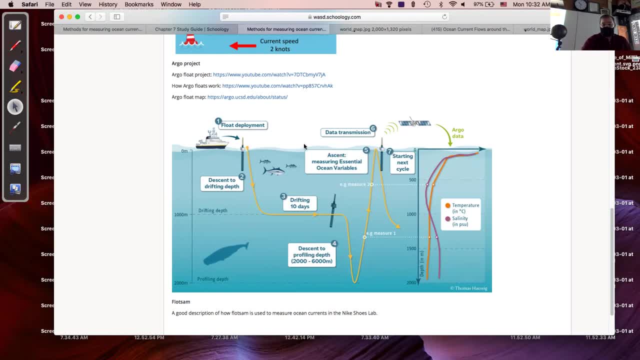 moving in some other kind of direction. So if all you ever do is just measure the surface motion of the ocean current, you don't get a full picture of the motion of the water at all depths. So there's this project called Argo. 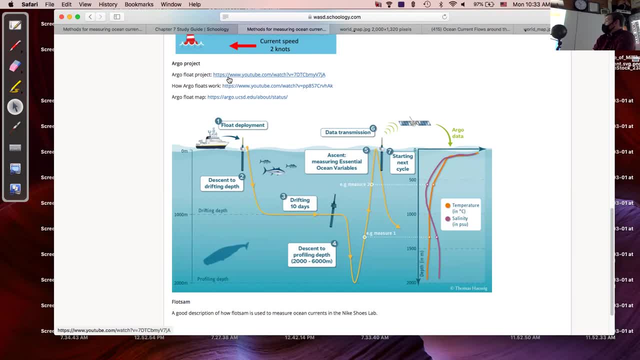 And Argo. there's a good overview Argo in that link right there. So if you're remote, this like Argo float project how Argo floats, you can see it: Argo floats work and Argo float map. I'll get to the map in just a minute. 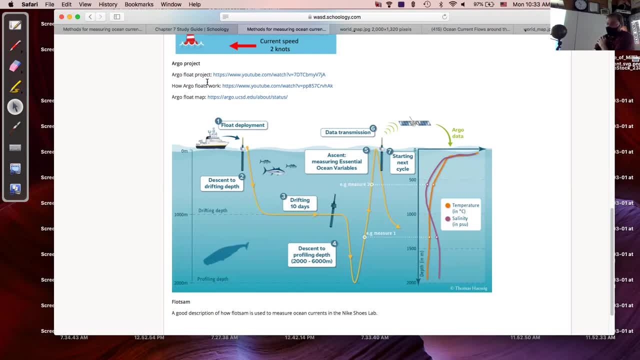 These two videos here I'll show in class right now, because they show like how the whole thing works and the ships and the whole get up and go. All right, this one's pretty good. It's only like, yeah, two minutes. Usually people have to be on their back to snore. 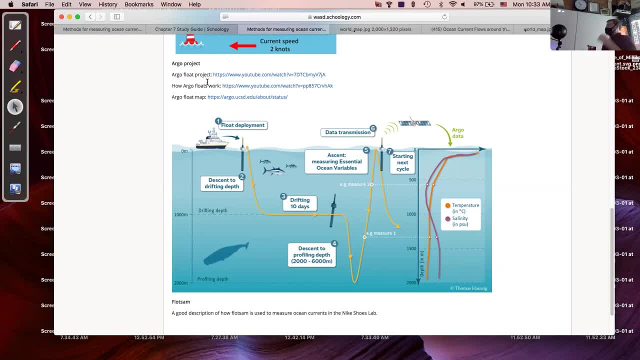 He snores like right, just like that. It's pretty savage. We know how to snore, So it's really good Thanks. Thank you very much, Walker, for your great analysis. It was really really really good, And thank you again for sharing yourности. 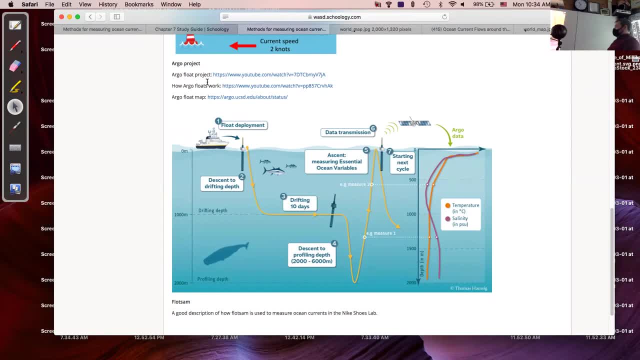 and thank you again for this incredible experience. I really enjoyed that, So we're really, really, really, really excited to share this with you And I'll let you know soon. But yeah, thanks again. Thanks again everyone. Bye. 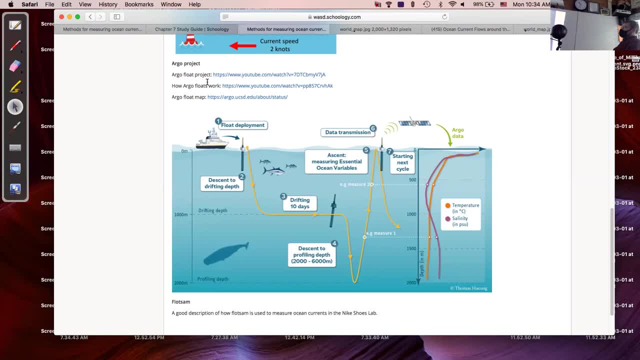 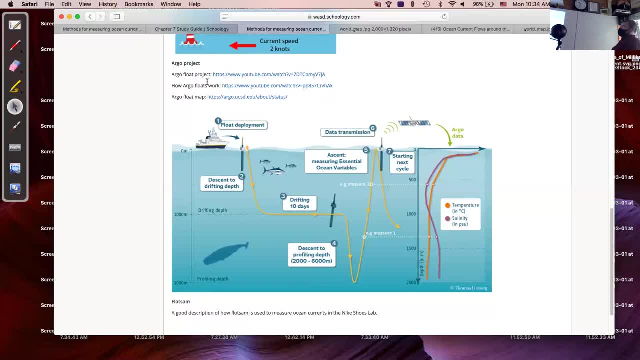 from every float you get the temperature and salinity down to 2000 metres. Basically the temperature is quite easy if metered with a thermistor, but the salinity is measured by measuring the conductivity really accurately and then, once you've done the temperature, you can use. 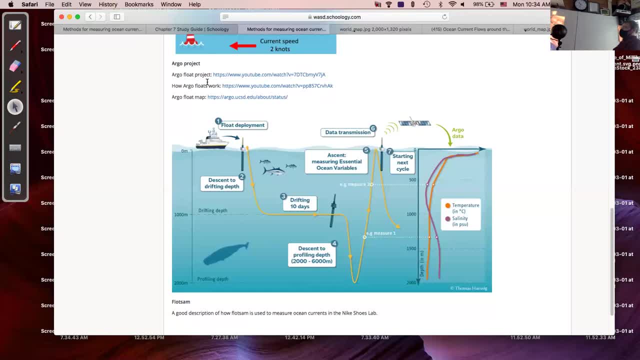 the conductivity to calculate the salinity. They're pretty high-tech instruments on every single Argo float to achieve that. That's a huge advance for physical oceanography and for oceanography altogether, because in the old days how you used to get that information was you had. 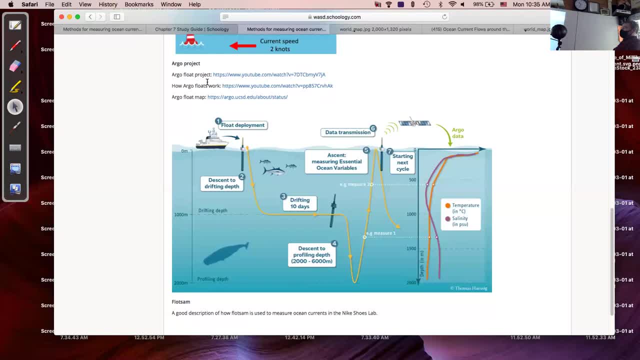 to take a ship out lower the CPD through the water column. It was very expensive and very expensive, whereas now you have this global network of floats and, since they report back by satellite, you have basically near real-time knowledge of the state of the ocean around the world. 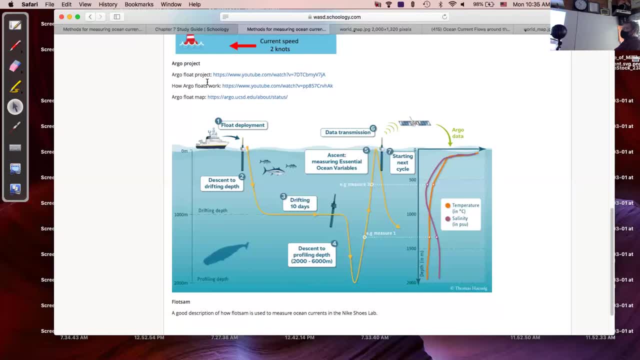 It's very hard to deploy floats in the southern hemisphere because they just aren't enough commercial ships to float floats up. So that's where these charges of Kāhiroa come from Now, at the moment there's about 3,700 floats all around the world and Kāhiroa to date has deployed 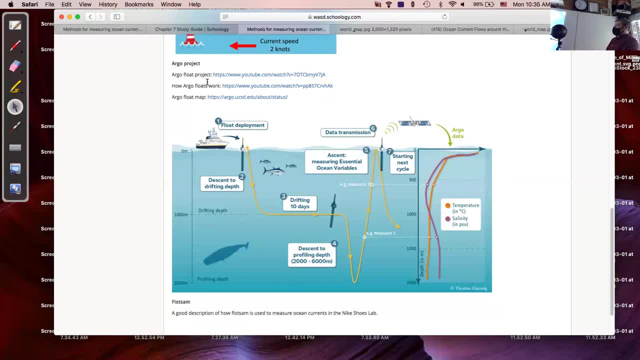 over 1,100 floats in the southern hemisphere. Without that we wouldn't have got floating Kāhiroa. So Niila and New Zealand really have been a big contributor to Argo and that's recognised around the world. Okay, Thank you. 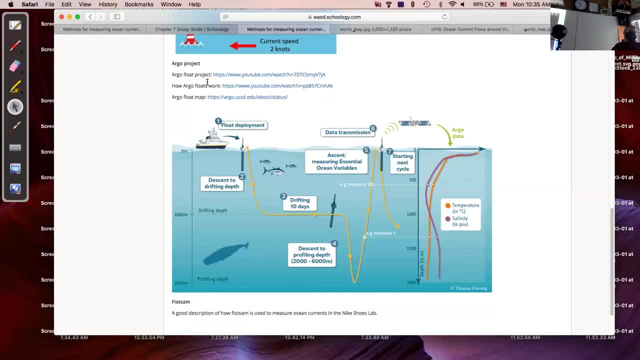 Nick, We have big gaps in our knowledge, particularly around how the biology and chemistry interact with physics and control things such as fisheries phytoplankton, which ultimately impact the way the oceans function in terms of productivity, the amount of food that they can produce. 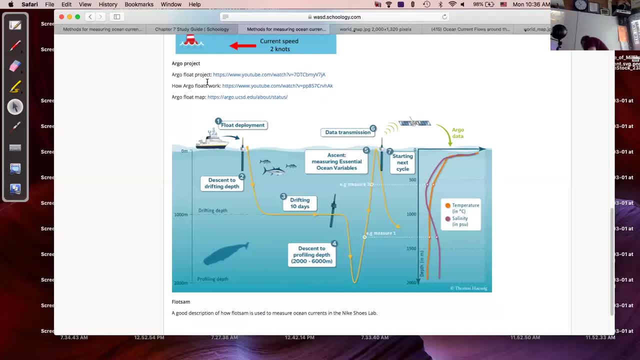 the way that carbon dioxide is absorbed by the oceans and take away to actually mitigate the climate change. So Anas' workload is like a robot that is operating free at sea. So it goes down to 1,000 meters, It sleeps for 10 days and after that it goes down to 2,000 meters. 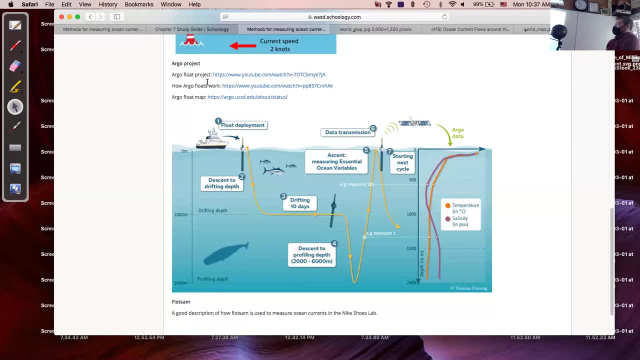 And while he is going up he is playing with the water. So he is making measurements of temperature, pressure and salinity up to the surface. When you arrive at the surface, it then transmits the data by satellite directly to show you. 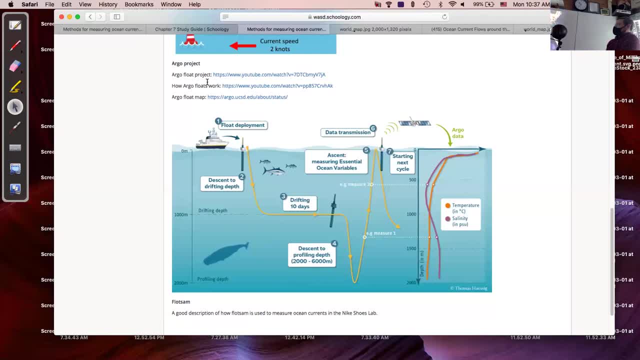 where the data are processed and delivered to the users. So what? General Lancer's project and what we've been involved in is actually creating better sensors that can go on these other boats, the so-called biogeochemical sensors that allow us to address biological and chemical types of the ocean, not just the physical. 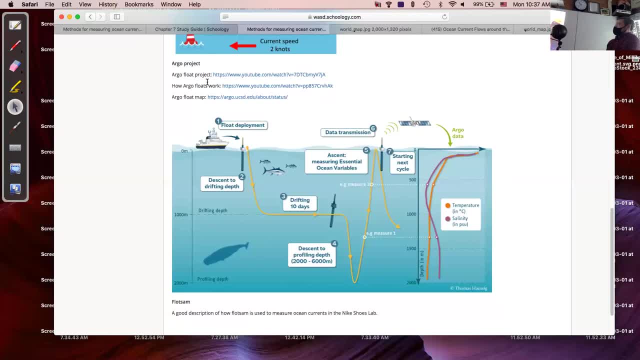 types. Our target is to have 1,000 of these robots operating globally in all the ocean, so that we can add a concrete picture to the ocean. What the Atlantis project has done is allow us to make a step change in our ability to observe the oceans. 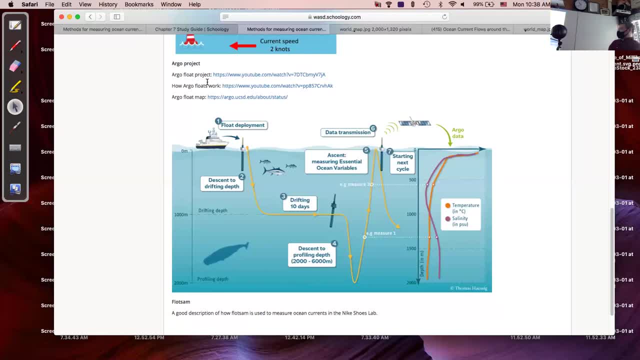 By augmenting the Argo system, using the Atlantis project as a pilot, we can show that we can observe our planet at a much better temporal and spatial resolution than we could before. All right, so the plan here. make sure that doesn't play something else. 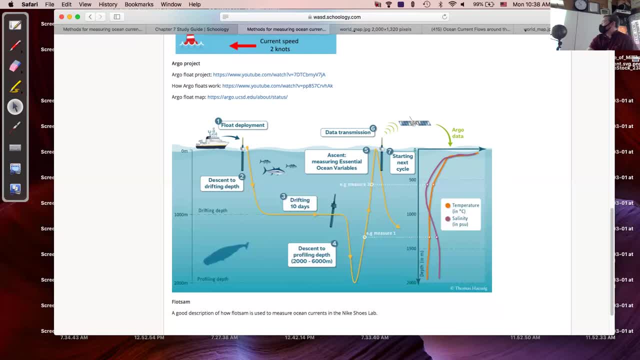 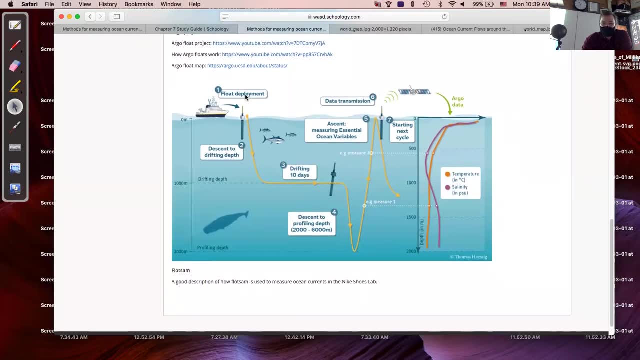 All right. so the plan is, those floats are deployed and because they have a satellite uplink, they can provide pretty much real-time data Whenever they submerge a float- Whenever they submerge, of course, they can't provide data, but whenever they come back. 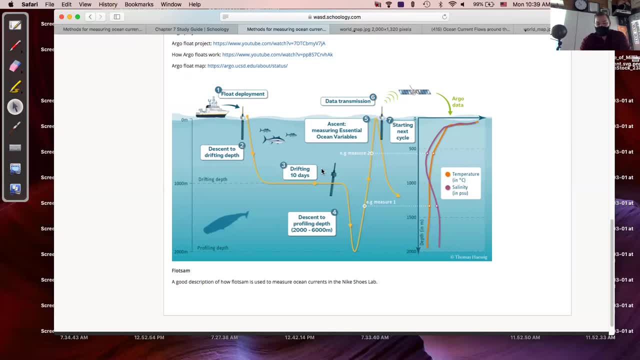 up. so you know where the thing's submerged, you know where it comes back up And how it varies. its depth is by taking water into a ballast tank. it makes it more dense and then it expels water from the tank and fills it with a little compressed air and 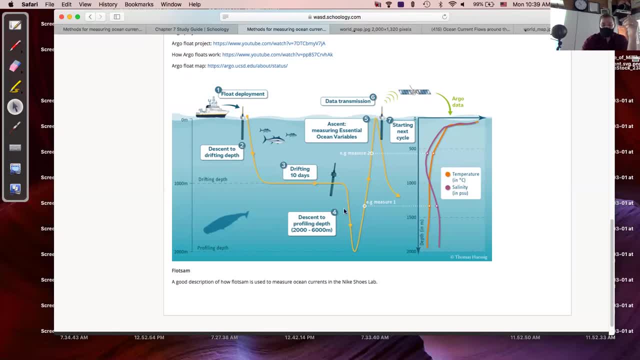 the thing floats back up all the while measuring differences in temperature on the way down, differences in salinity on the way down and back up. The bio Argo floats also measure nitrate and phosphate concentration And, uh, uh, magnesium and calcium in the water, uh, which give you a better sense of. 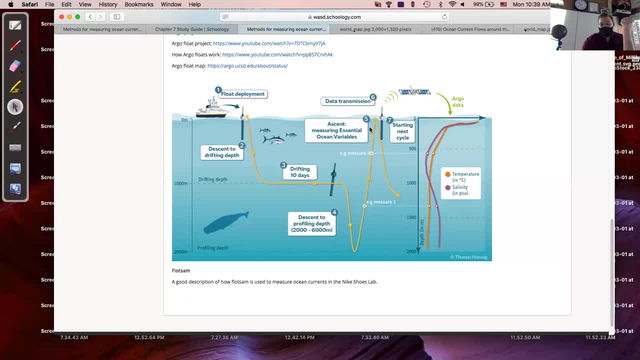 differences in chemistry on the top and bottom And they can be serviced. So whenever you know where the like, whenever it runs low on battery power or it needs to be serviced, you can find out its location because it has broadcasted GPS signal. but 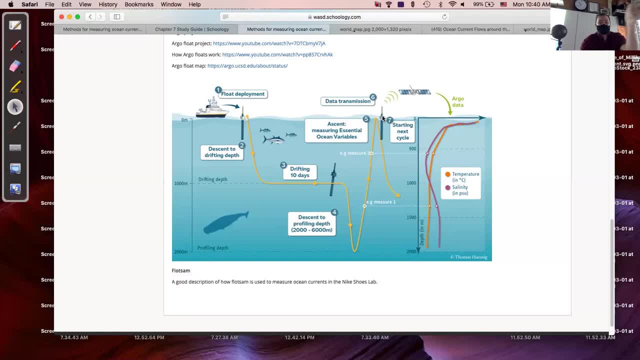 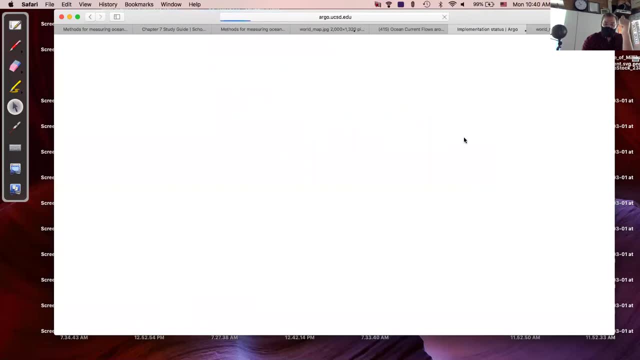 also has a small radio transmitter on board that you can just track the same way as you'd like track an animal with a radio tag or whatever like that. So here's the current. So here's the current Argo float system. So this is the. this is the Argo status. 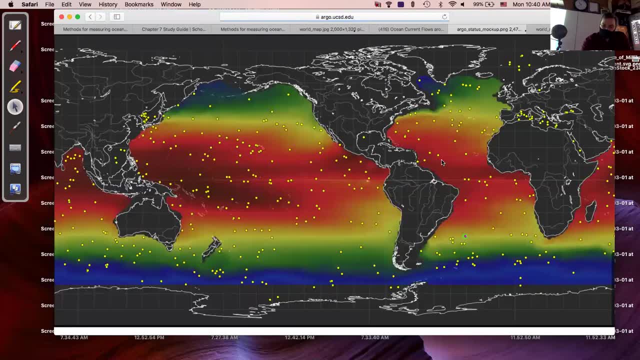 Let's see. So these are reported locations in the last three days. So this is all the Argos. Those are those floats that are deployed around the world's oceans that have reported their location within the past three days. So this is like the newest data itself. 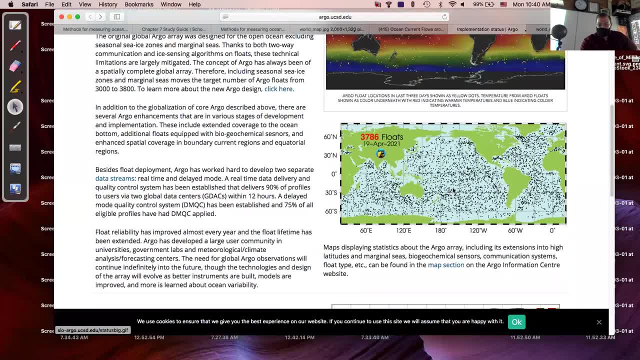 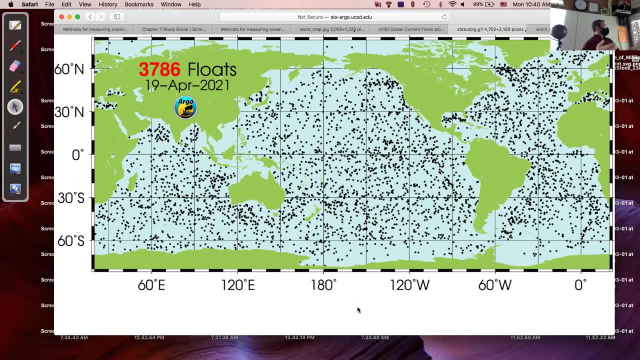 It's not a hot clickable map, But this one shows the current- uh well, the current- location of all the ones that ought to be out there. So there's a total of 3,786 active floats. That's uh April and that's today. 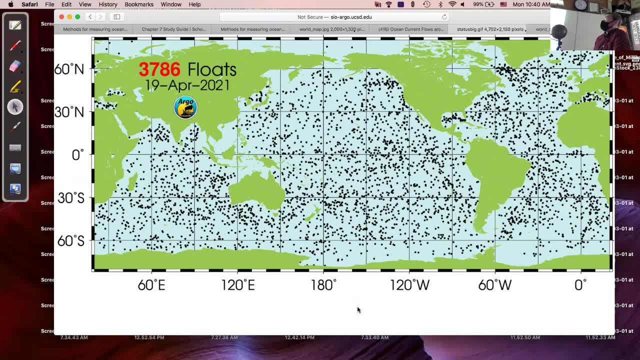 And those are the relative location of all the floats. So, in a way, uh, oceanographers around the world are able to know current temperature salinity data from all those floats. And when they said that there are customers, just as an average person, you don't have. 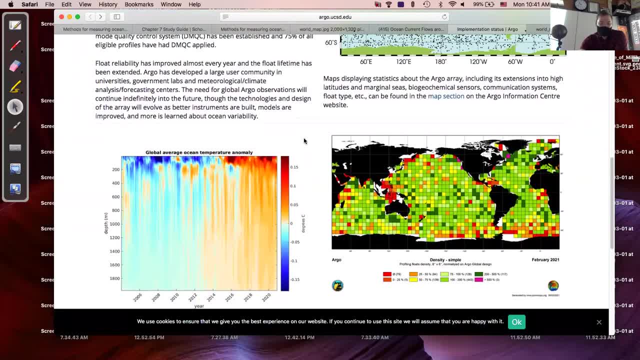 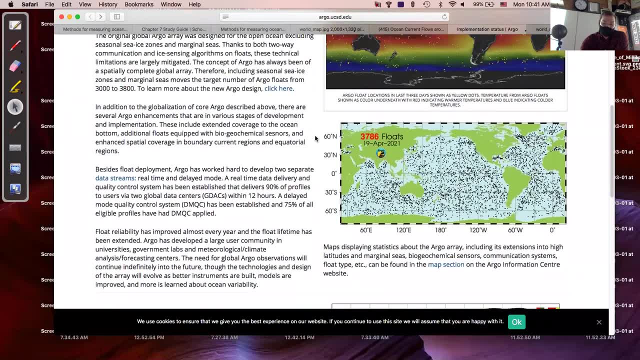 access to that data. but world oceanography organizations like NOAA uh can get information, uh people who work in fisheries. So, like, if you're a large fishing, like a company that does uh offshore fishing, you want to be able to get as much data. 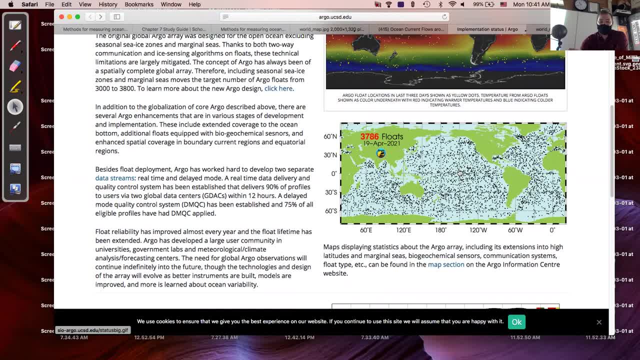 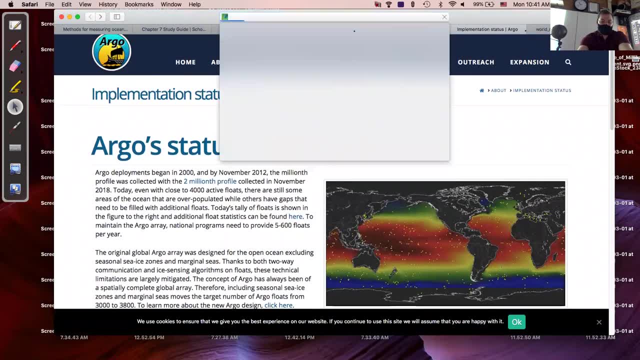 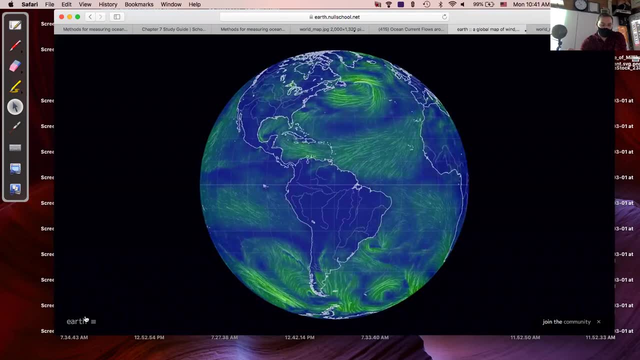 As you can, to inform where you should go to find the greatest amount of catch using the least amount of fuel, And then, whenever you're at uh earth dot null school, the way in which this site is able to display current and temperature information. 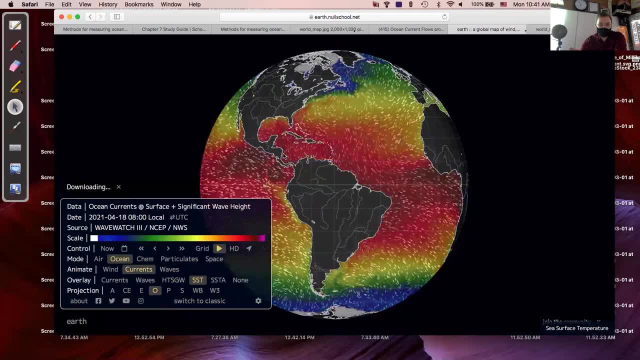 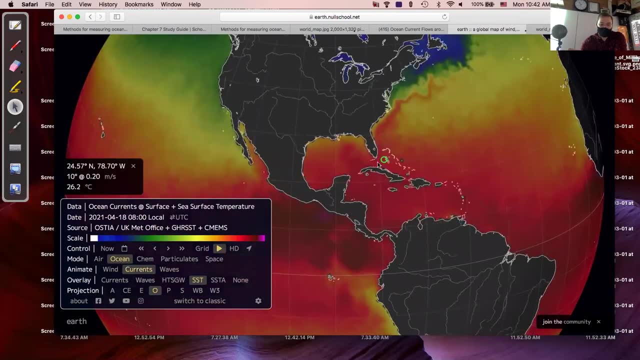 So when you go to ocean current and sea surface temperature, whenever you're on this site and like you see, you know, whatever the temperature of the water is, The sea surface and the direction of the ocean currents, how it's possible to know. 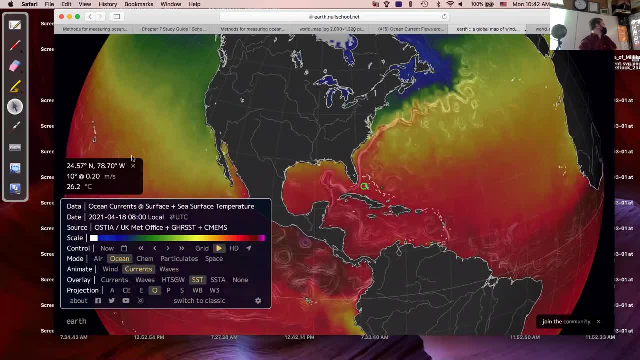 this information in near real time because this has uh. let's see what the data is. This was as of uh eight Zulu yesterday, or eight universal coordinated time yesterday, So that's only like a day old data in terms of ocean temperatures and current direction. 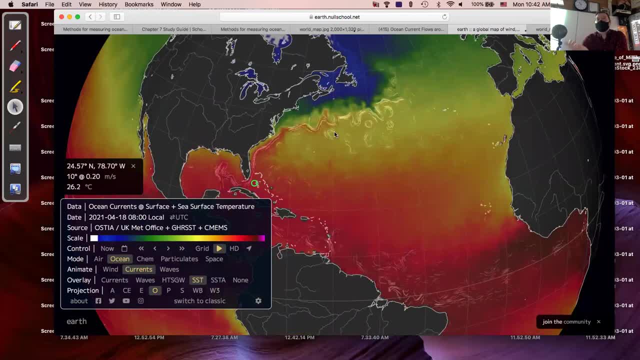 and speed information. Okay. So what you're seeing is that that data comes from the uh Argo uplinks. So you've got autonomous robotic temperature, salinity, depth, current measurement uh probes that then send their data up to satellite. 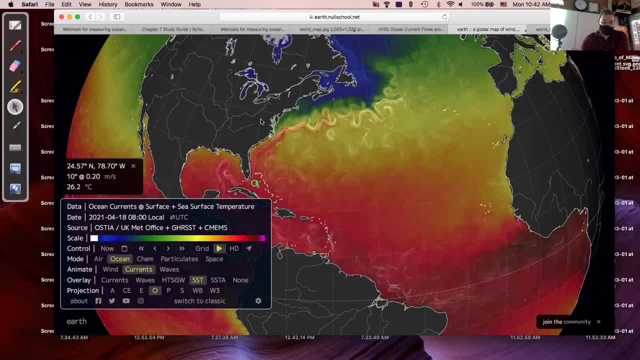 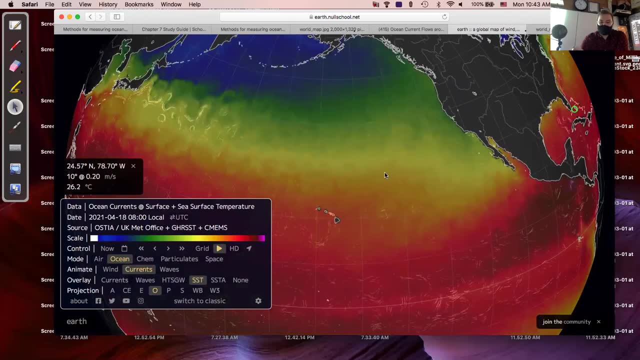 Those satellite downlinks can then be used by oceanographic organizations and also be used to be able to see this, this information, in real time. So you can't see the granular data, In other words You can't know as just a regular consumer, what the last position of an Argo thing was. 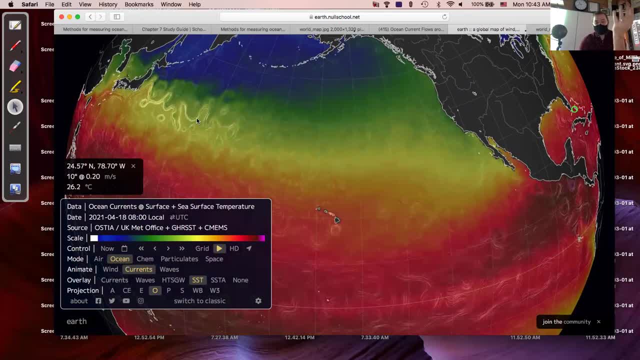 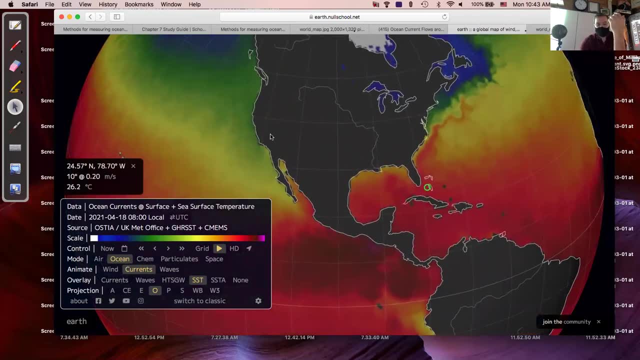 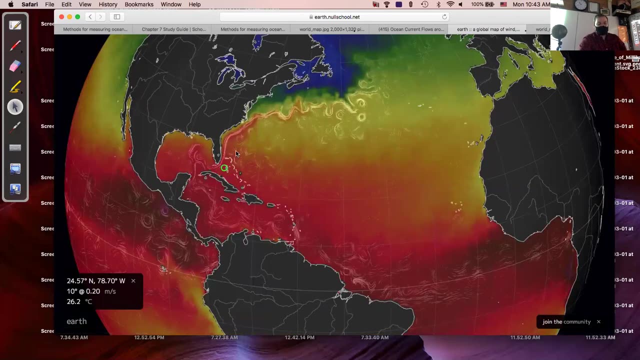 if you're not a subscriber to the network, but to the general public. there's a good overview information. It's also used by meteorological organizations to figure out, like you know, the propensity for an El Nino event to take place or, uh, you know, if you're trying to do some kind. 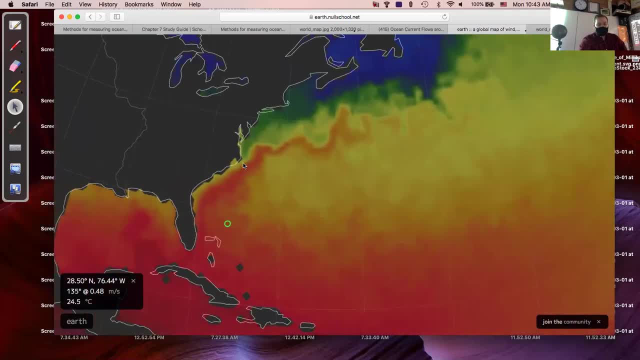 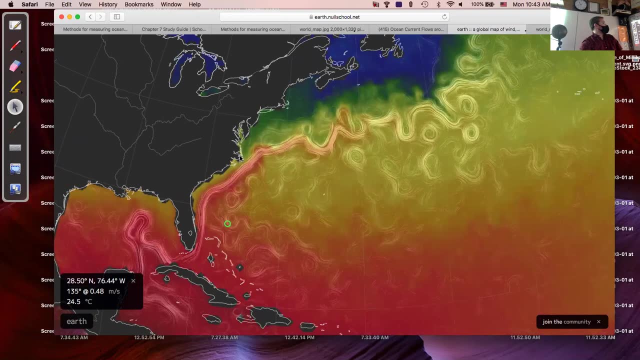 of weather forecasting, maybe here, North Carolina, uh, and you're quite you're a little bit unsure about what the coastal temperature is going to be. What would be useful is to see, like, what the speed of the Gulf stream is because of the 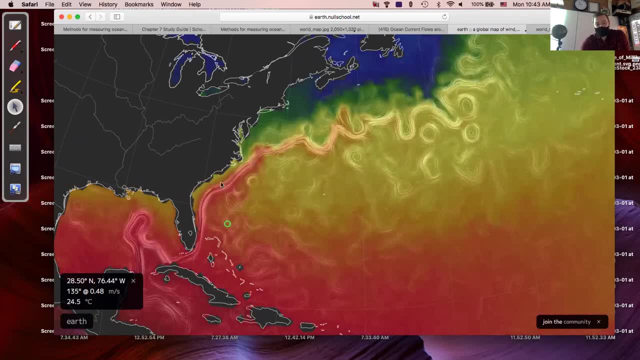 Gulf stream is relatively fast, carrying a high volume water, and it's expected to increase, than that would encourage the temperature here to be higher. If, instead, you're at a period of time with the Gulf stream uh having a reduction in speed or reduction in current, you would expect the temperature here to be relatively lower. 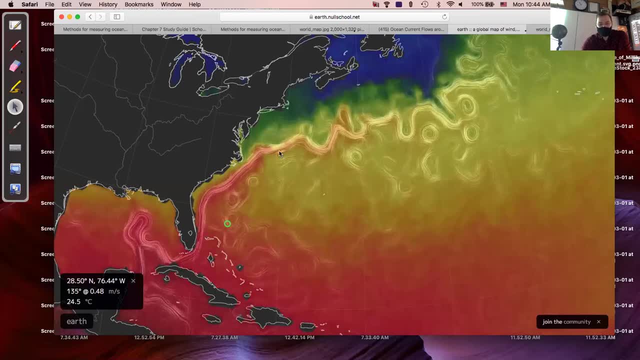 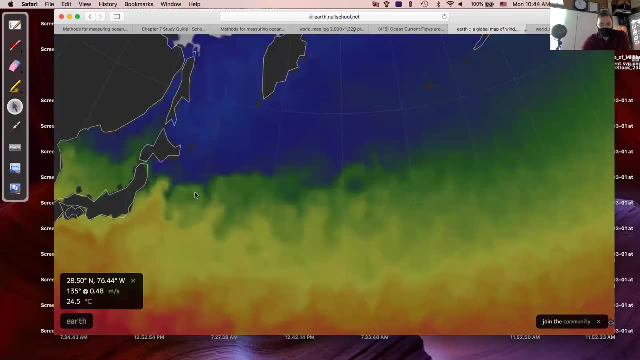 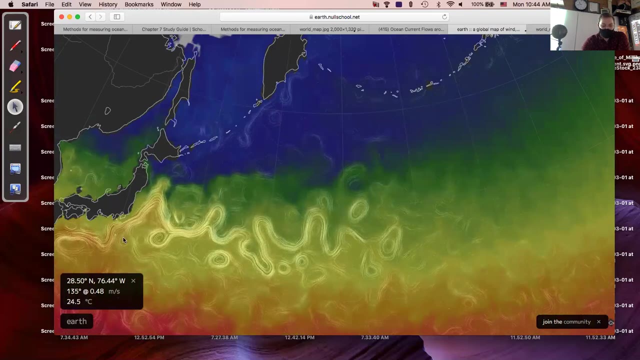 Cause there's a lot of heat that's delivered by the Gulf stream or maybe on the West coast. Uh, the Japan current famously flows. It's called the Japan current because there's a cold current which flows from Japan. Well, it's actually pretty slow up along the Aleutian islands, but there's a relatively 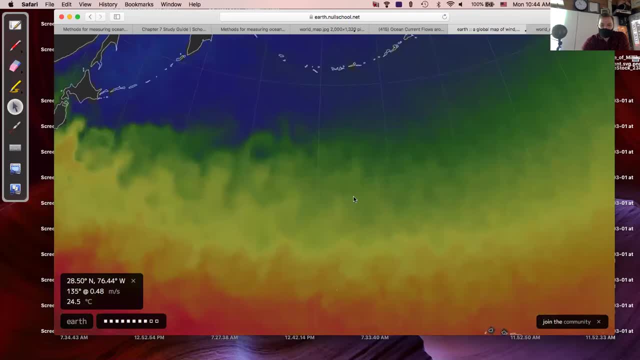 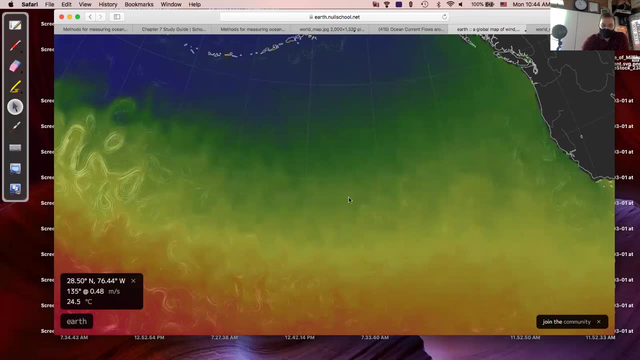 cool water current which is cooled by the North Pacific as it comes across the Pacific ocean toward the West coast of the United States. It's actually pretty diminished right now. Okay, And that's what keeps the water relatively cool on the West coast, because all that water. 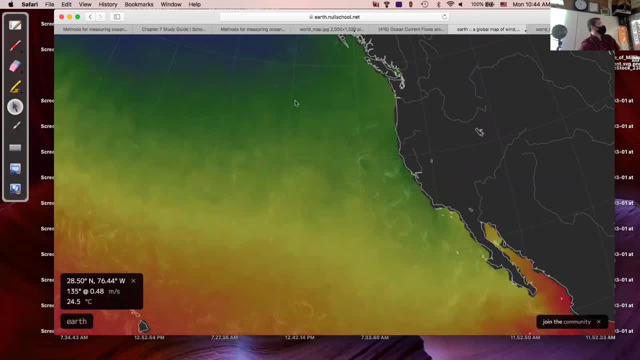 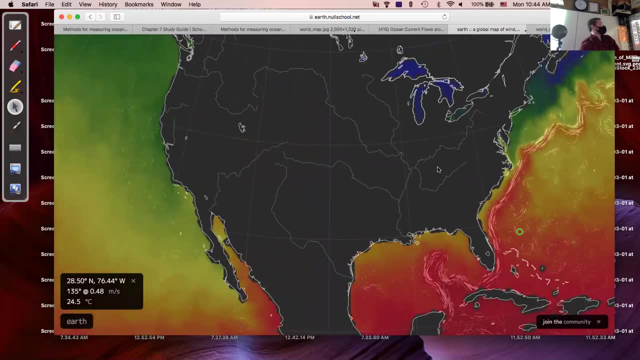 has spent a lot of time in North Pacific, traveling across the North Pacific toward the West coast of the United States. That's why we have comparatively cooler temperatures of the water on the West coast compared to the East coast And also much milder uh currents on the West coast right now as compared to on the 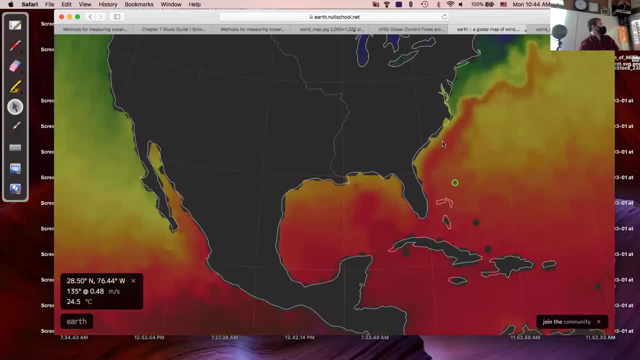 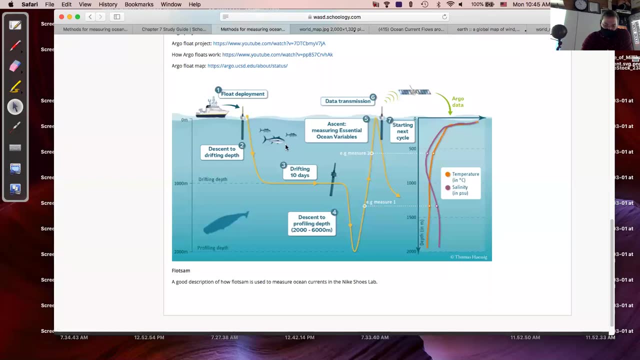 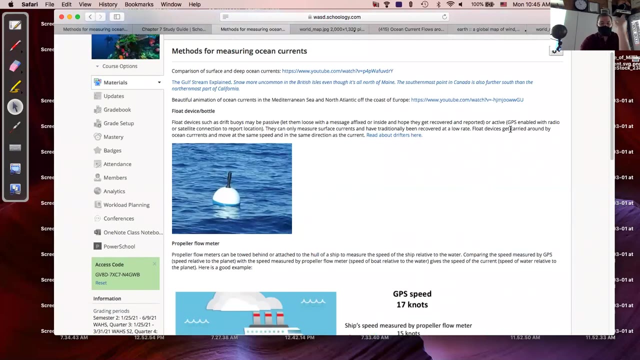 East coast. This is a pretty fast Gulf stream speed right now. So those are the major ways in which, Uh, ocean current speeds are measured. The the last like example: So you actively measure ocean currents using intentional float devices or bottles which 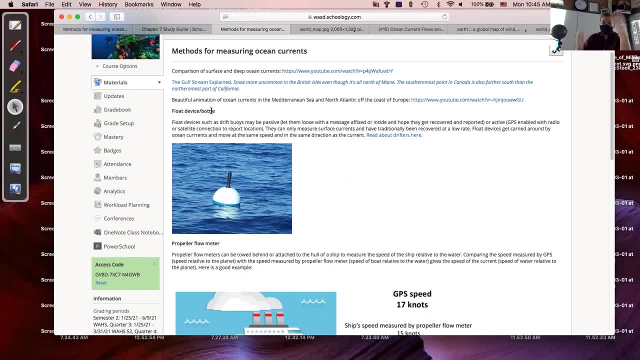 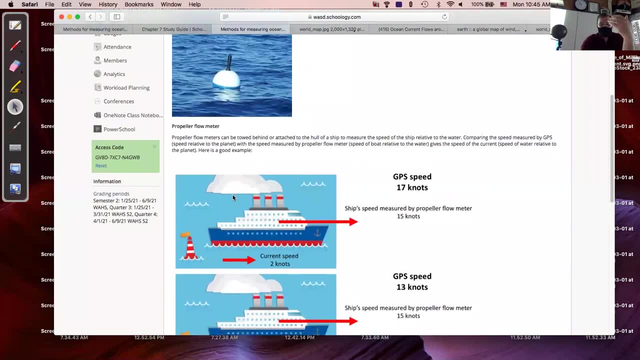 you say, Hey, here's the location of the speed or here's the location of the time and date when I dropped the thing off. Then you pick it up or you find it later and have it broadcast. information on the surface. You can measure speeds of currents on the surface by comparing the speed of the boat. 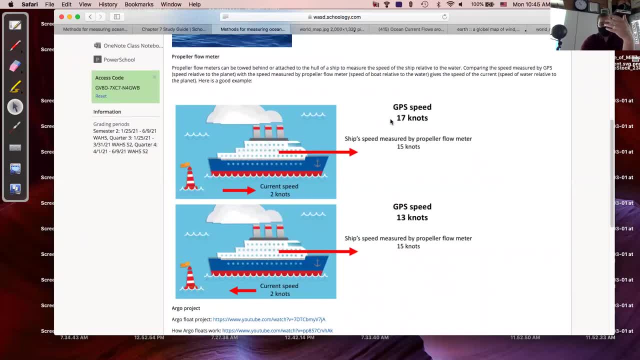 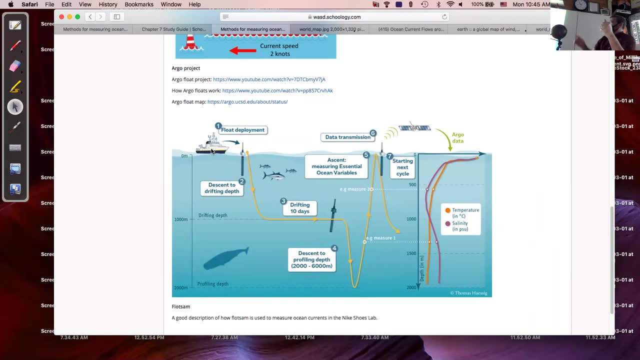 relative to the water, to the speed of the boat relative to land? Uh, and derive from that like what direction and the speed of the current must be? Argo is the most expensive and sophisticated things. A lot of times those floats are deployed, uh, sometimes they can be deployed on research. 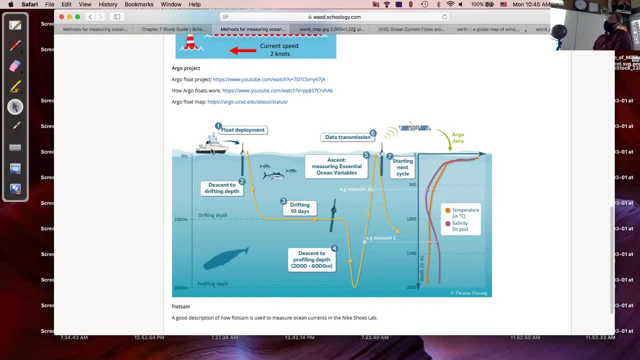 vessels. but then also like, if you're in NOAA, the National Oceanographic Atmosphere Administration, and you want to deploy another 15, uh, you know- Argo sensors, you may contract with a fishing fleet and say, Hey, you guys are heading out from, maybe Seattle. 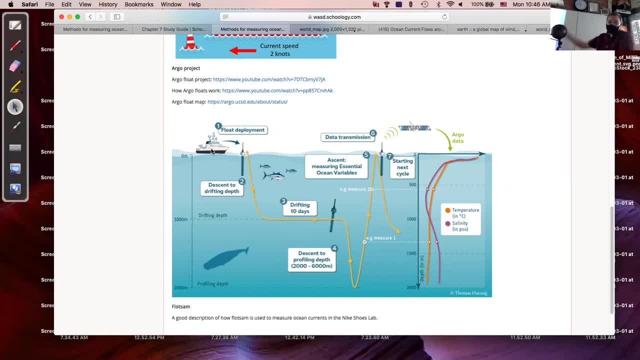 You're heading out into the Pacific Ocean to the approximate location where we want to deploy them. Then, on board the fishing vessel, they may have scientists who are, you know, going to do the deployments. You're like, Hey, while you guys are out there doing your fishing and hitch a ride, we're. 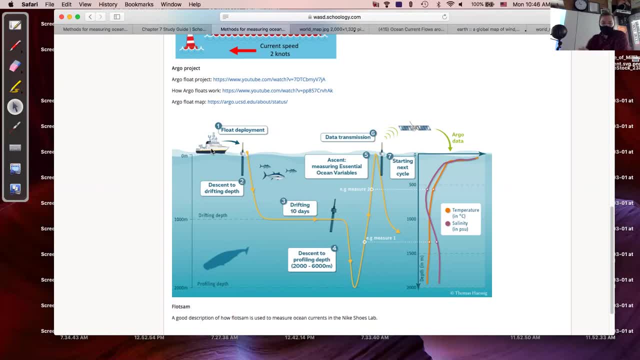 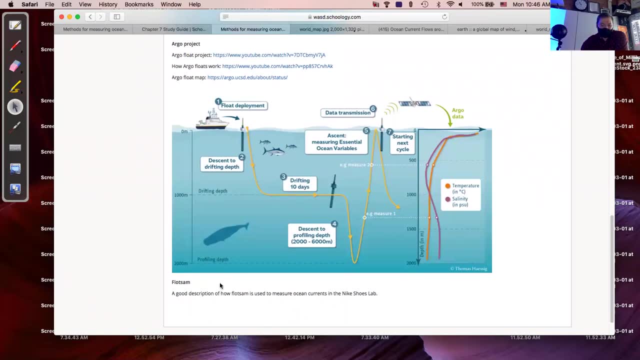 going to throw so many things in the water And then you just bring us back to port, like whenever you're done, Because, uh, research ships are very, very expensive to operate. The last method is the unintentional measurement of ocean currents by flotsam, like in the. 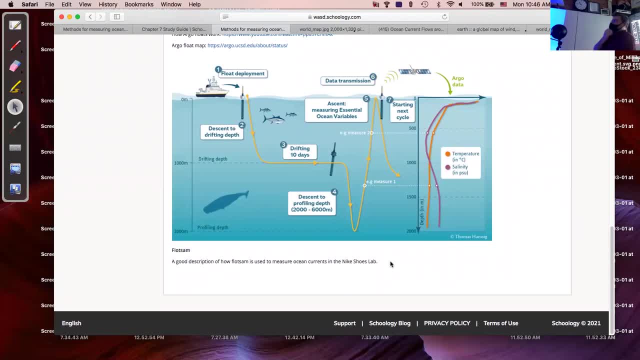 Nike shoes lab to just say, Hey, sometimes some crap ends up in the water. Maybe it's trash, Maybe it's stuff that got thrown overboard off the ship. We know where and when it was released. And then, uh, tracking the position of motion that stuff lets you know about, uh, let you. 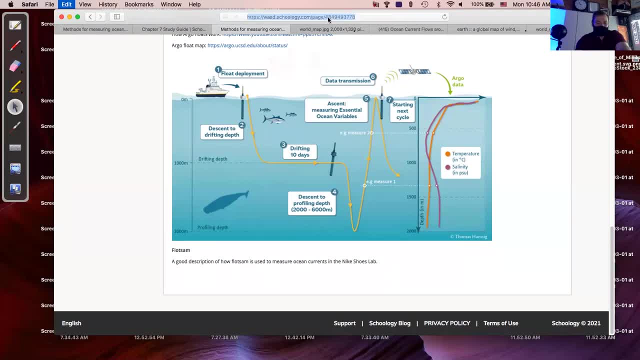 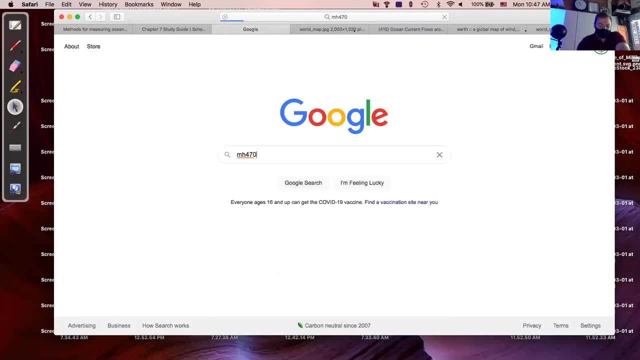 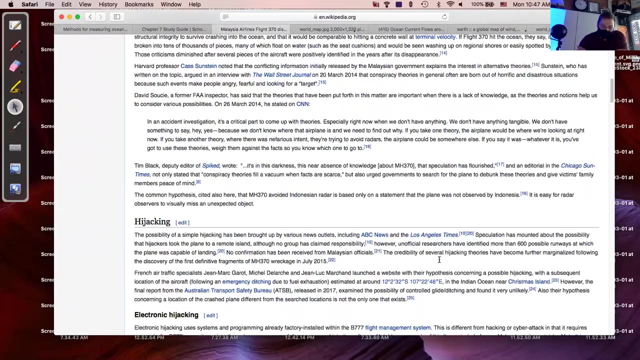 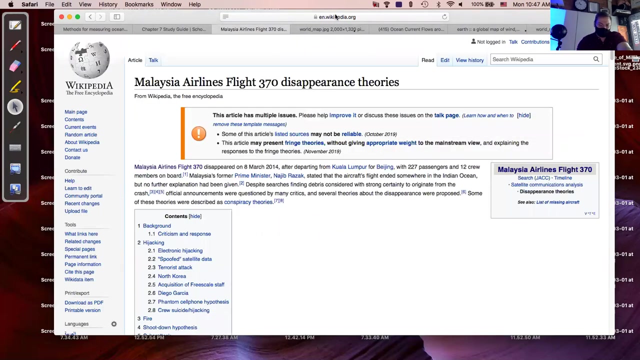 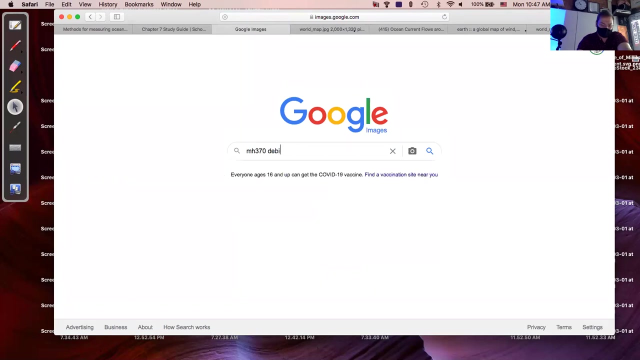 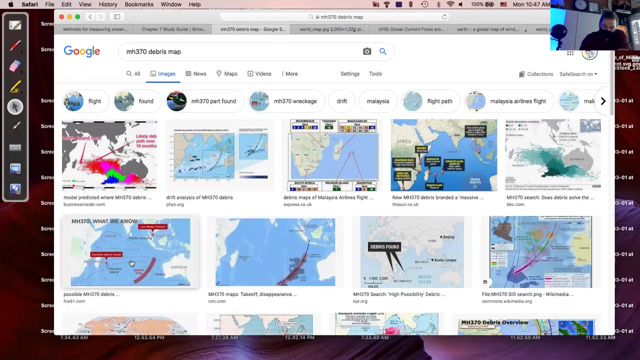 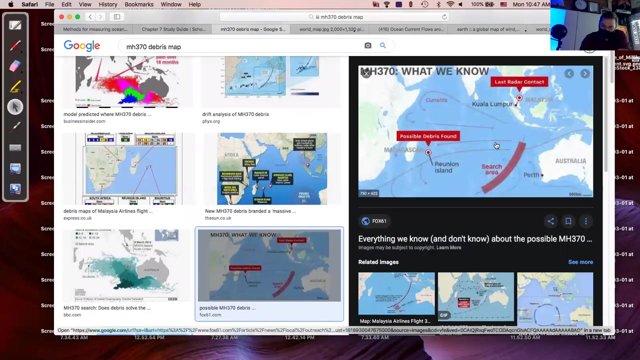 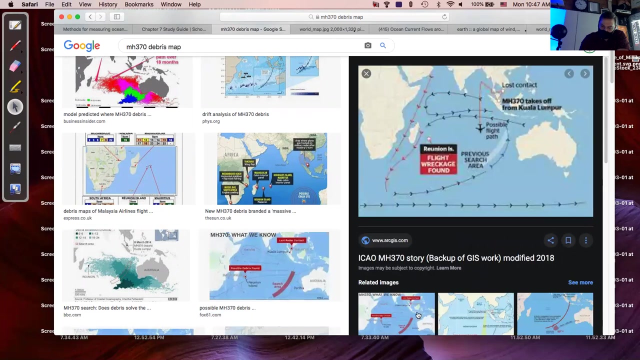 know about the direction of the currents. Okay, Um, another example. So, mage, was it 470?? I think that's the number 370.. Let's see what we're finding. I guess that one's okay. Yeah, So I mentioned this before this came up. I don't know in what context or whatever, but 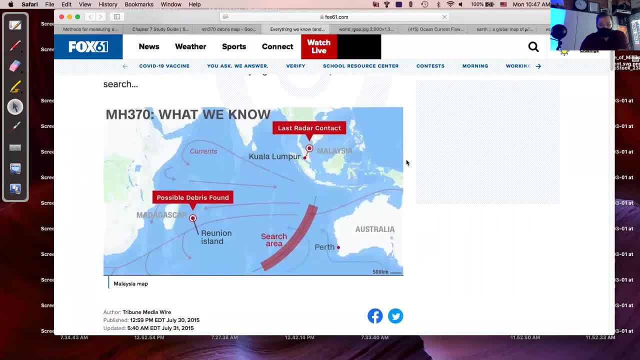 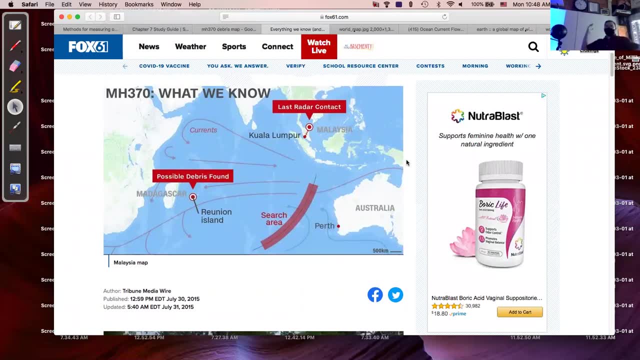 there's a maybe about ocean depth and how broad the ocean is. There is an aircraft- a Malaysian airlines aircraft MH370, which just disappeared quite a few years ago And uh, so it took off from Kuala Lumpur, Malaysia, heading toward the Northeast lost. 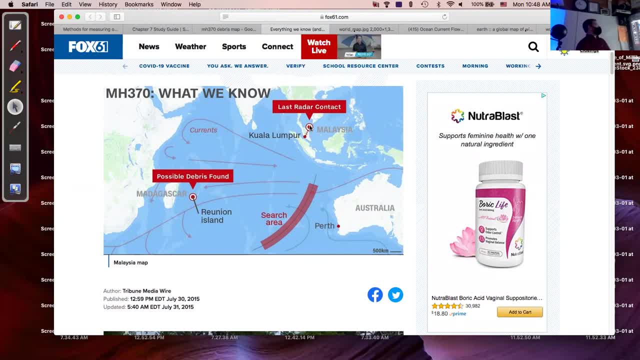 radar contact here, But then there's a good probability that it crashed or it crashed in the ocean somewhere along this path. That's from data, from satellite uplink, from engine monitoring information, And there's some debris that was found off the coast of Madagascar. 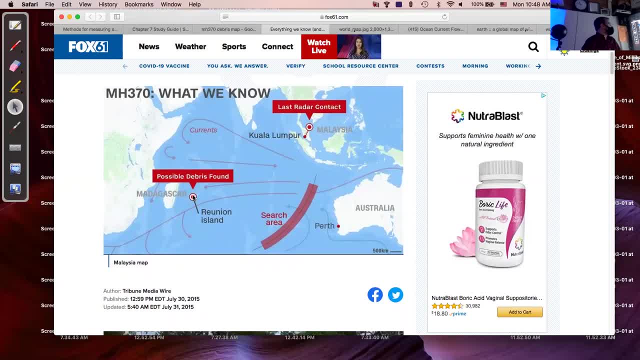 Uh, Reunion Island, which is from that aircraft. This is about six years ago. it washed up And that makes an awful lot of sense because if the plane crashed into the ocean in this region here, which is like the northernmost part of this possible search area, uh, debris. 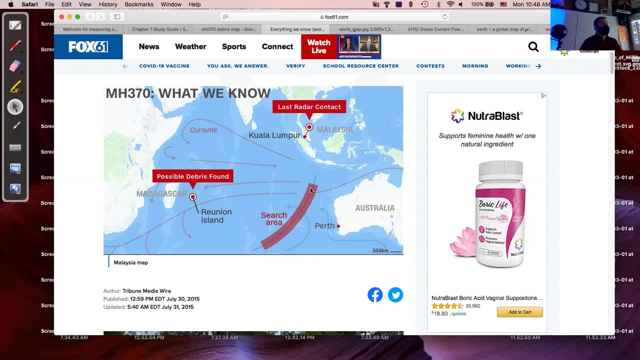 on the ocean surface, seats, quotation devices, any kind of uh passenger effects that float on the ocean, uh that floating debris will be carried by ocean traffic. It will be carried by ocean currents. There is an ocean current which has uh, you know, through between uh, between the Micronesian. 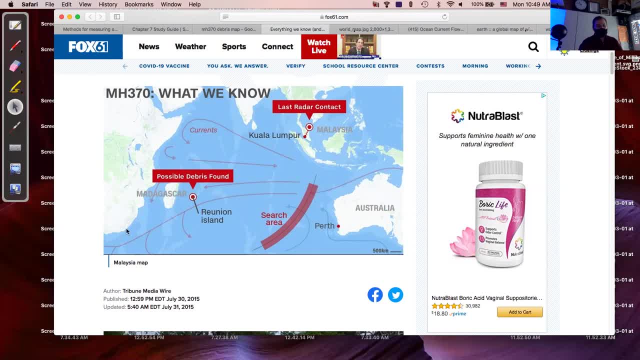 Islands and Australia heading toward the West, heading toward Madagascar and then going down around Southern Africa. But, uh, debris from this is likely to continue to wash up, uh, along Reunion Island, Madagascar, the West coast of Africa, And the more debris you find. 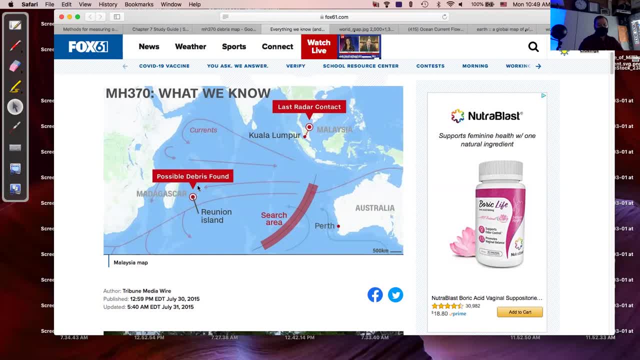 And if you're very sure about the location and the time that it washes up, it gets you better information about the possible location where the plane went down. Unfortunately, even if the plane went down down here, it's possible for the debris to 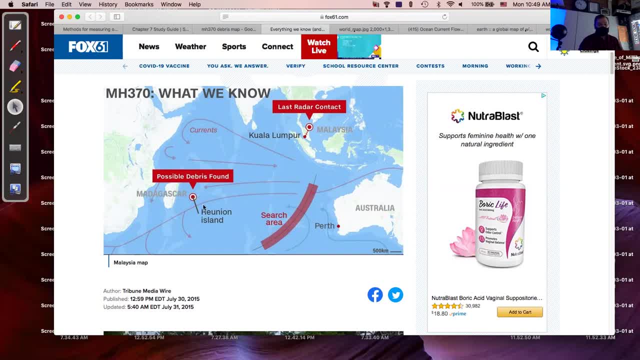 end up there because of the current which flows up to the north and then to the west. But if you know the speed of the current and you know the relative time it took for the and the absolute time it took for the uh debris to move, you can determine like a probability. 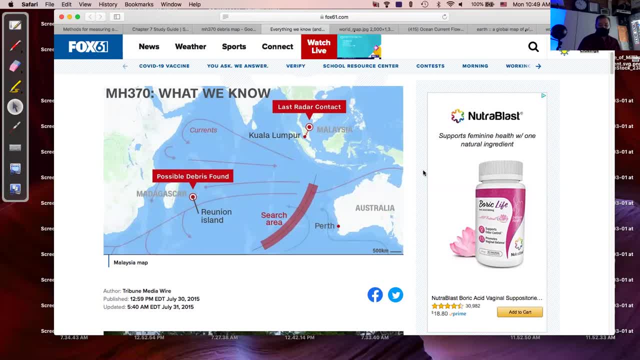 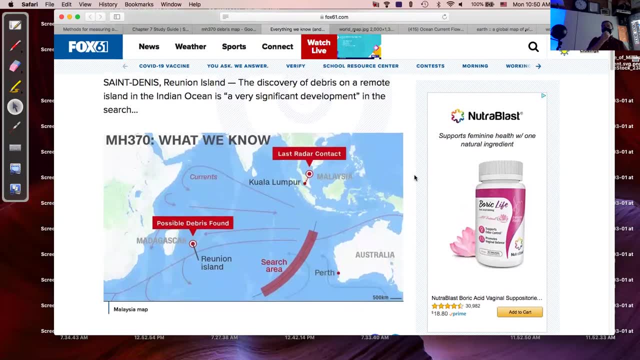 of where the plane would have crashed along that, along that location. It's possible we may never find, uh, that plane, but it's also possible that it will be found. The problem is, when an airplane hits the water, particularly at high speed, uh, most of it ends up. 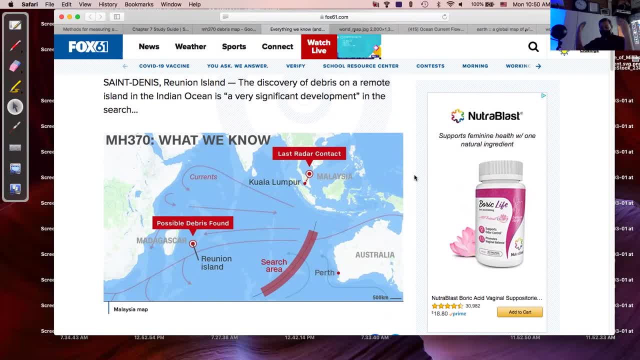 just getting broken up into lots of little pieces, and most of the stuff sinks the ocean floor. So you're not looking for like a big long fuselage of an airplane That's not going to still be intact. Instead, the whole thing's probably going to be all uh broken up. 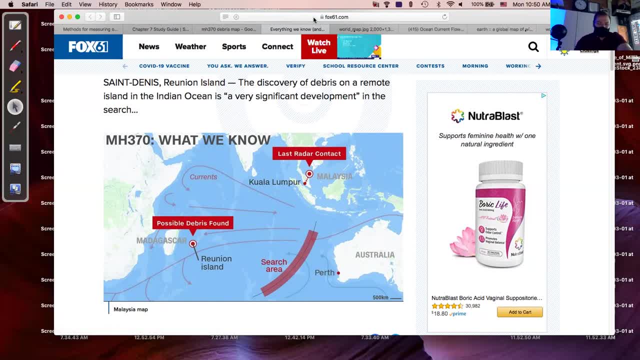 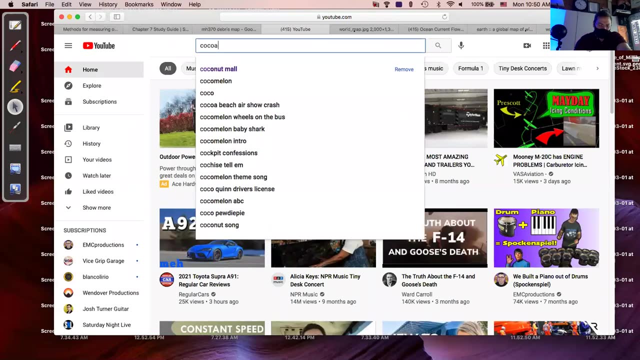 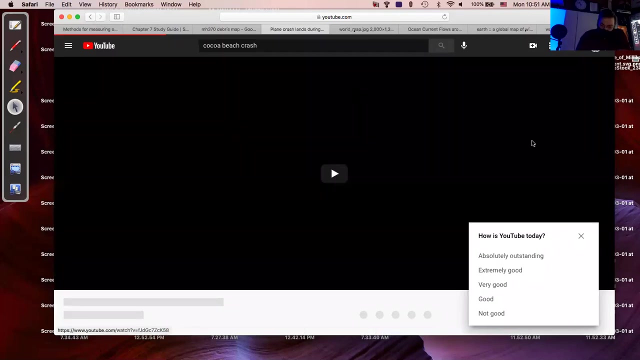 So I don't know if you saw, this is kind of it's unrelated, but there's a uh pilot who had to ditch a plane off Cocoa Beach yesterday And he's okay. But Cocoa Beach, Florida, uh, there was an air show and it was mostly like older aircraft. 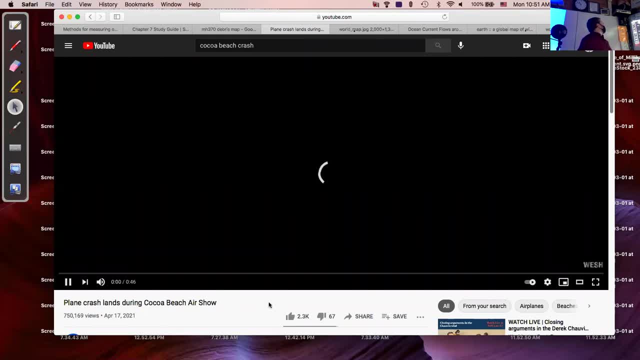 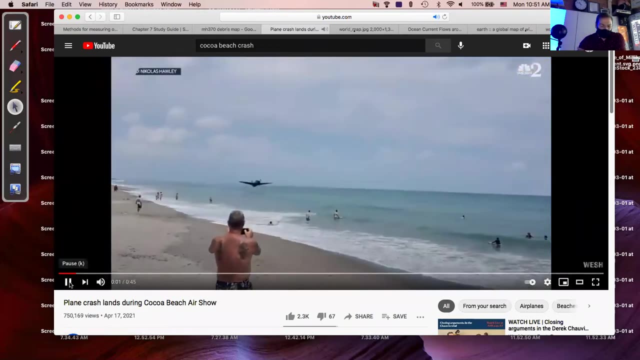 And this is a uh TBM. It's a plane that was used as a uh dive bomber, torpedo bomber, navigation aircraft in World War II and then after World War II, And the pilot ran into trees And he ran into trouble. 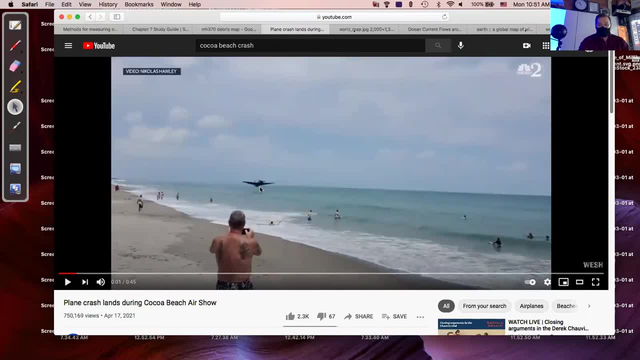 So here's the plane. The pilot ran into trouble and it was too low, Couldn't make it back to the airfield, So he needed to ditch, And the only reasonable place to ditch was on the beach or in the water, And the beach was like full of people. 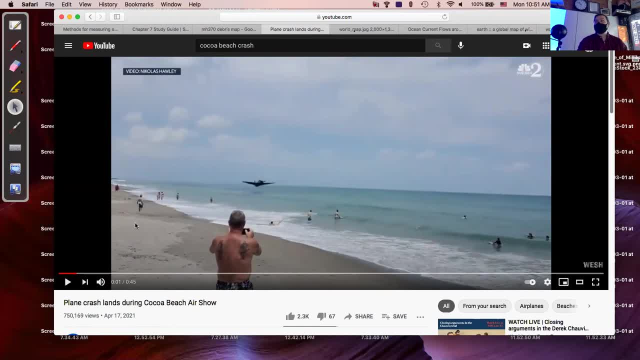 So you're. it's really disappointing when people are like sunbathing and then you hit them with a plane. So you're trying to like. the pilot has to make a quick decision as to how to uh put the plane down somewhere. 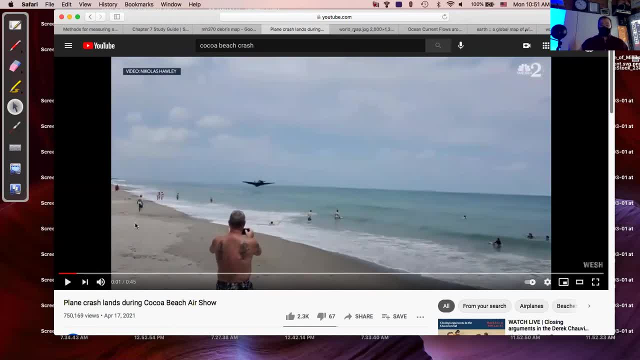 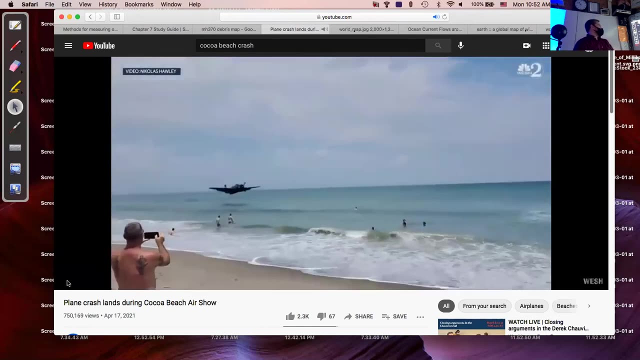 And the pilot is as safe as possible from people on land and as safe as possible for the pilot himself, And then also try to consider his own rescue and the possible salvage of the airplane. So this is about as good as you get. He came in and then look there's like people right here, right. 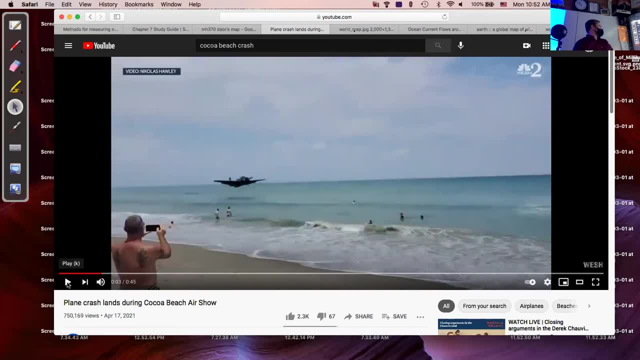 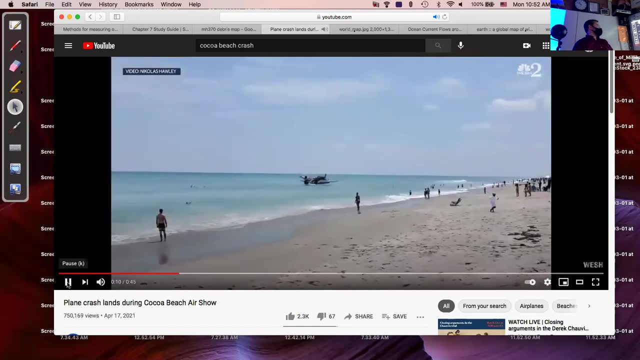 Can you imagine being out swimming and then this plane's like this And you're like what the heck is he doing? so low? And the pilot ditched the plane, Uh, flew right over there. Uh, flew right over the heads of some people and put it down. 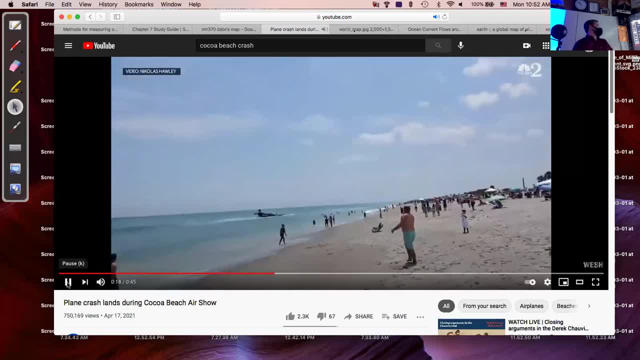 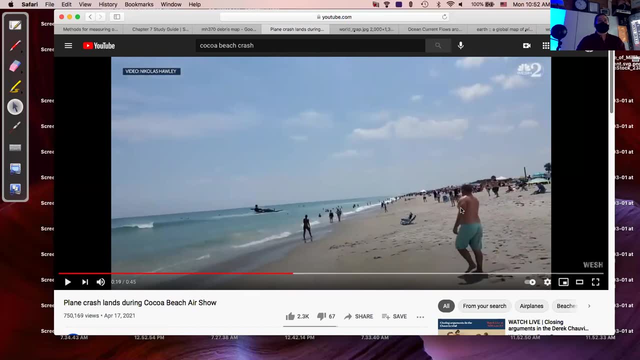 And then the pilot was okay, Got out and they salvaged the airplane. Look at the beach: full of people, Isn't that nuts? So it's the right thing to put it in the water, Like if the beach was empty of people. putting it on land would have been a good idea. 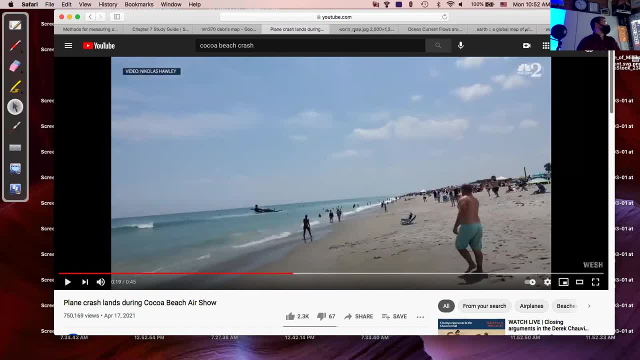 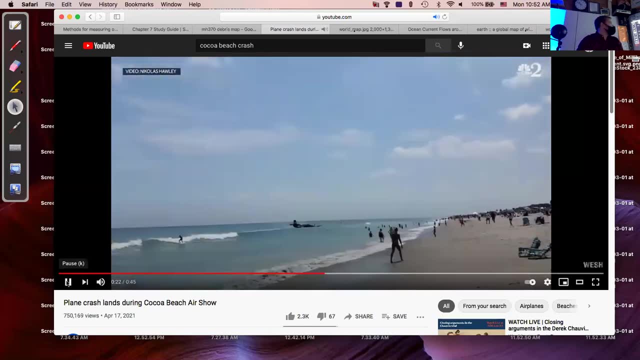 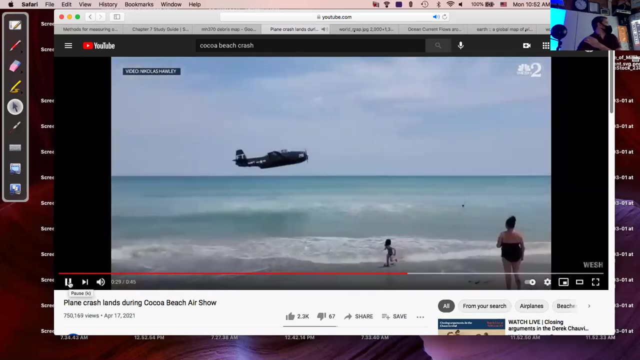 He could have just belly landed on the sand, Except if he would have brought it down where people are here. he would have just killed a couple dozen people or something like that. But yeah, he made it. He was okay. Yeah, So this, uh, this plane, the TBM is uh. well, when I first heard it was a TBM, uh, and it went down in the water. 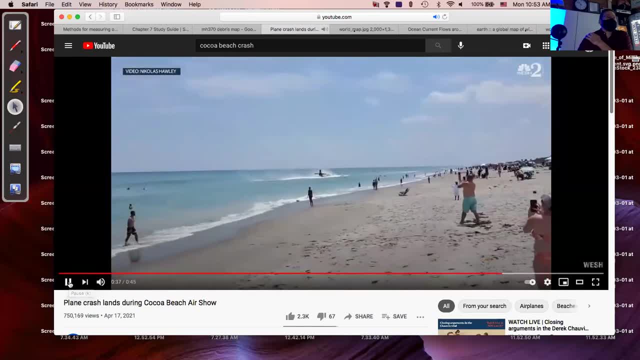 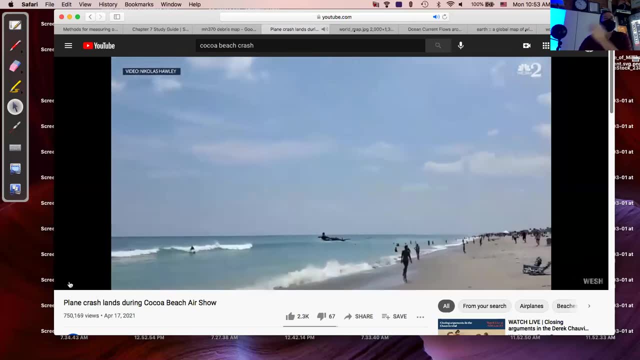 First thing I thought of was: well, I know a famous case of that. Uh, president George HW Bush, the first president Bush. he ditched a TBM, the same plane when he uh, when he was a pilot, and he survived. 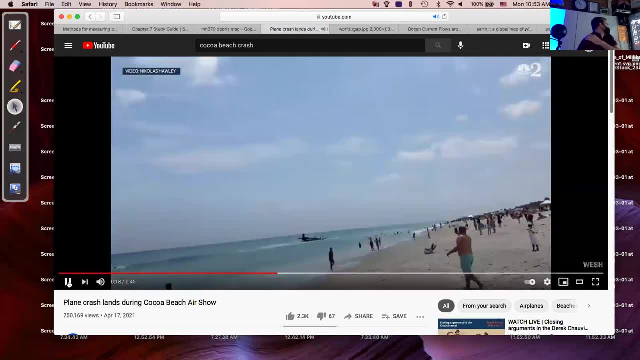 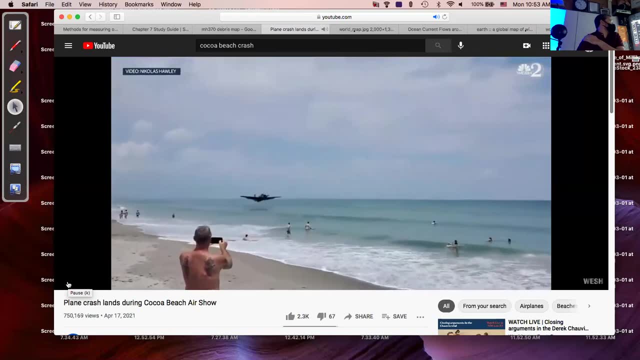 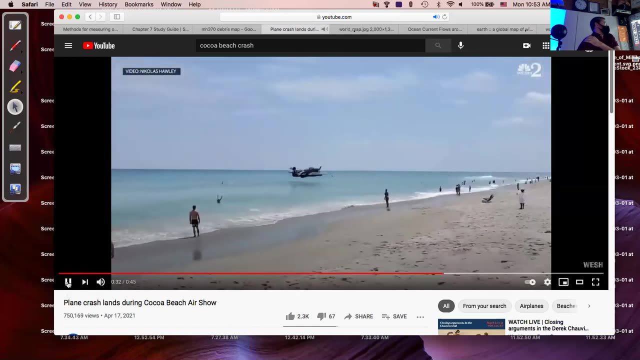 The other two members of the crew passed away. But if it's not survivable to water, land a TBM and we wouldn't have two of the presidents we've had, because both George HW Bush and his son, George W Bush, uh, wouldn't have been presidents. 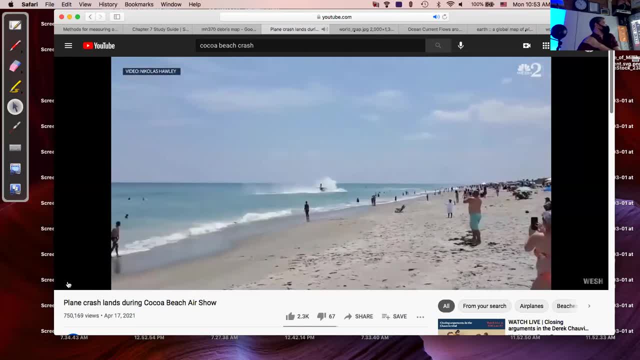 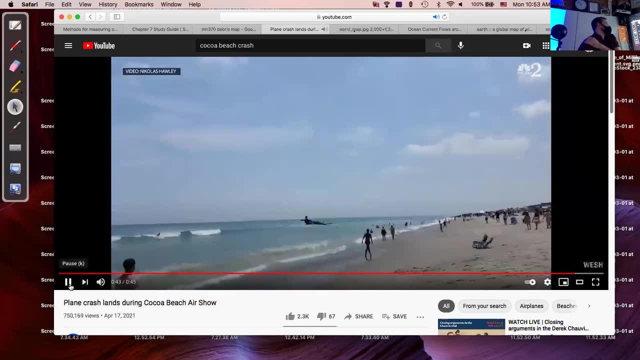 President, George HW Bush, hadn't survived the crash. So, yeah, that's common in the plane. It goes down real quick, but this was in real shallow water So they were able to secure it. They'll haul it back up. They'll be able to recondition the plane.